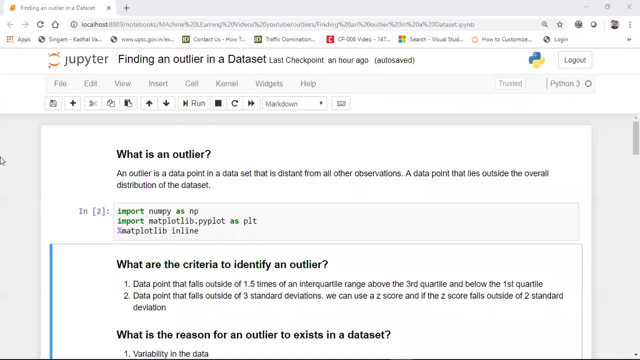 Hello all. today we'll be discussing how to find an outlier in a particular data set. First of all, to begin with, guys, outliers are important also for some of the use cases, and it may also not be important for some of the use cases. So let me just take an example. 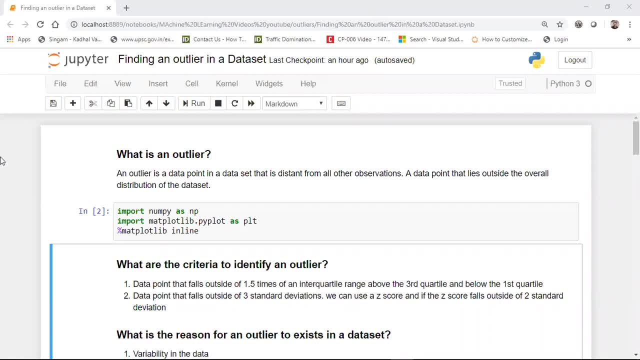 Suppose, if I have a use case which is called as credit card fraudulent data set, Now in that particular data set you'll be having some kind of data which will act like an outlier. You know some of the transaction which will be actually fraudulent- Those information. 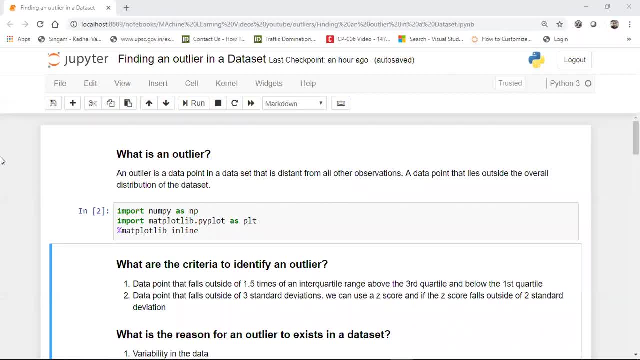 are very, very important. In that case we can consider that that particular outlier is very, very important. But in the case of normal data set, where we have, due to some human errors, that particular data has been captured not in a proper way, you know so. 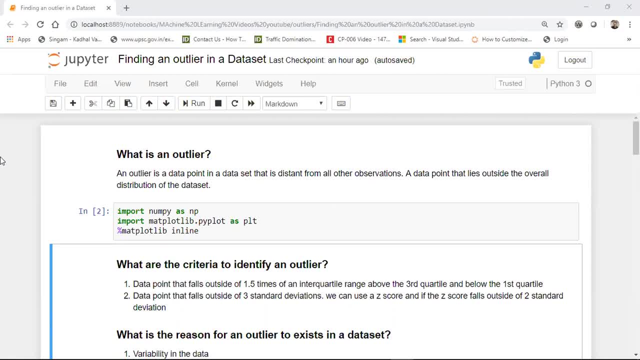 that rare value can also be an outlier which is not useful for our data set itself. So, first of all, before I move this ahead, make sure you watch this video till the end, because I'm also going to show you some practical implementation: how to detect an outlier in. 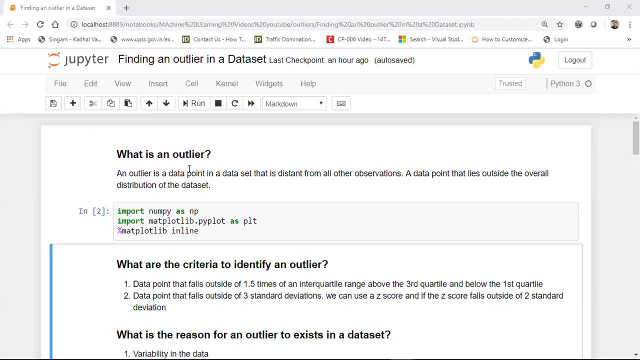 a data set itself. So first of all, to begin with, what is an outlier? See? outlier is a data point in a data set that is distant from all the observation. That basically means that it does not belong to the observation that is actually present in the data set. You know it has a distant. 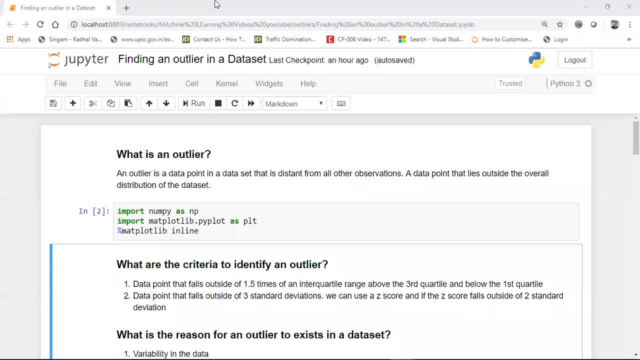 characteristics, in short. So let me just give you an example. Suppose I have some data set over here. Okay, In my x-axis I have some value like weight. In the y-axis I have some value like height. Now, usually what happens is that you know, I have some value like 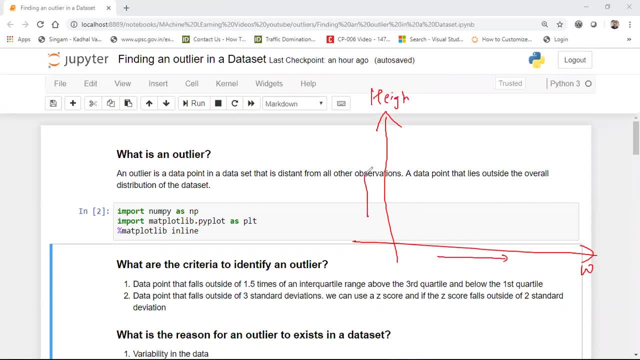 weight, You'll be seeing a scenario that, as the weight increases, your height also increases. Most of the scenarios like that, But in some scenarios you'll be seeing that, even though the weight is somewhere here, our height will be very, very high. So this: 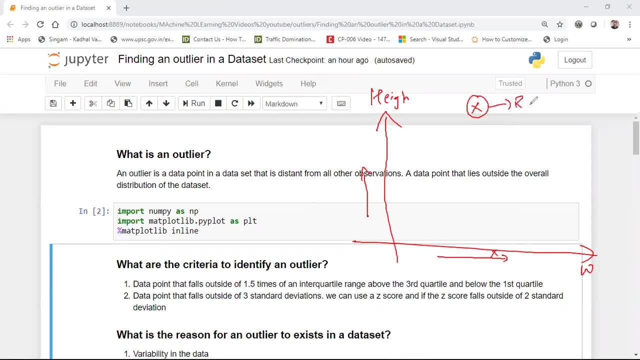 is just like an outlier, you know, and this is a very rare condition, very rare condition Specifically, you'll not have those scenarios in a population data set. Okay, So this is just one example. Now, if I take an example of credit card fraudulent data, you know, 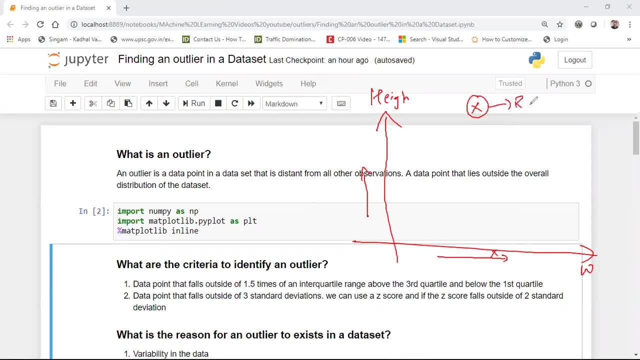 is just like an outlier, you know, and this is a very rare condition, very rare condition Specifically, you'll not have those scenarios in a population data set. Okay, So this is just one example. Now, if I take an example of credit card fraudulent data, you know, 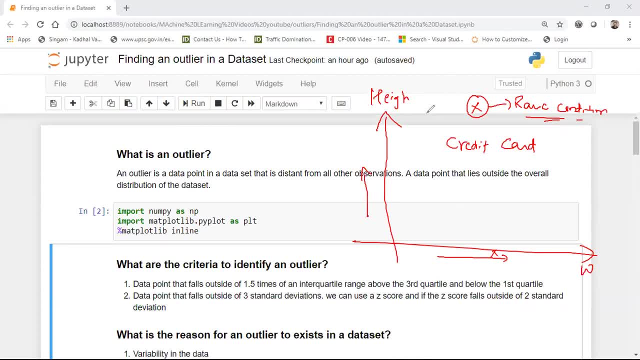 credit card fraudulent data, In that you'll be seeing that the weight of the data set will be very high. You'll be seeing that some of the transaction will be very rare. You know some of the transaction which is just like an- uh, you know- fraudulent data. 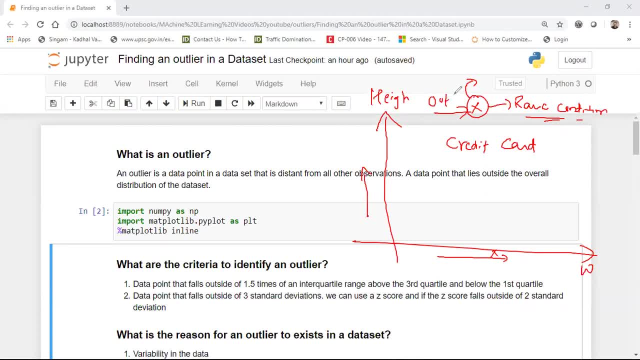 will be very rare, And that is what is the most important. outlier data right. So there are various ways to handle this kind of outliers and this kind of outliers that are rarely present, If I take the example of heightened weight. Okay, So they are different ways in. 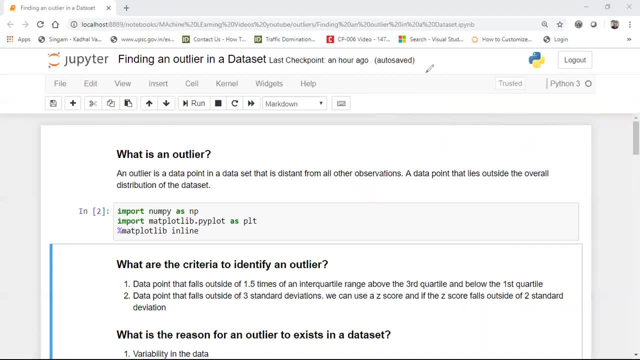 this particular video we will be specifically seeing that. suppose, in a data set due to human error, there are some data that is got captured as an outlier. How do we find that particular outlier? It's that Okay. So initially, to begin with, I'm going to import some of the libraries. 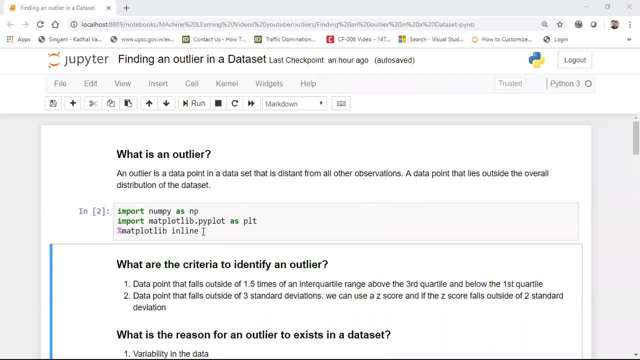 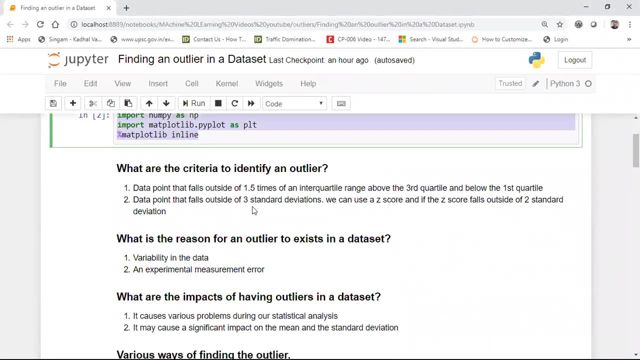 like NumPy, Pandas and Matplotlib. Sorry, Pandas is not there. NumPy and Matplotlib will be sufficient. Now what are the criteria to identify an outlier In this particular video? I'm going to show you two different techniques. One is with the help of something. 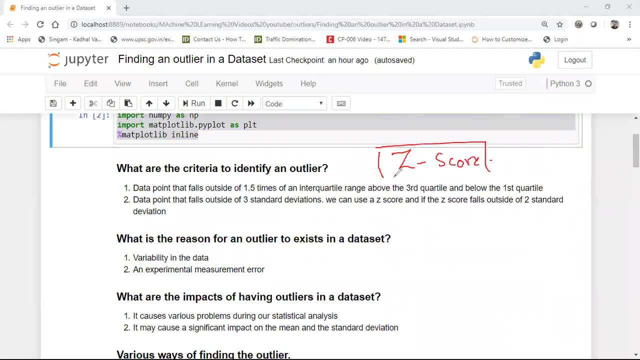 called as Z score. If you know about standard normal distribution, I think Z score will be very, very easy for you. This again, anyhow, I'll be explaining what is this Z score? Then the next thing is something called as intercontinental range. Okay, So we are going to discuss these two techniques. 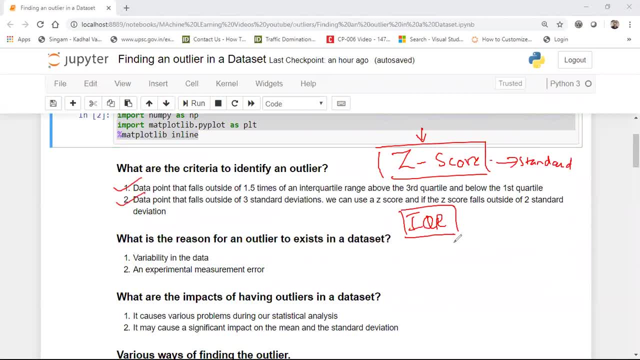 The first one is basically the intercontinental range. The second technique is something like the Z score. Okay, Now, what exactly Z score that we need to understand? Always remember, guys, whenever we have some data set. let me just take one feature and 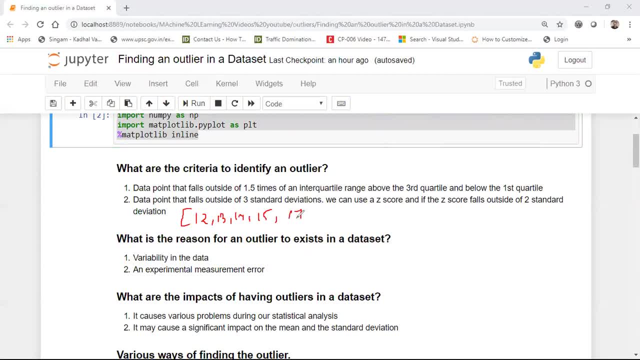 I have some data set like 12,, 13,, 14,, 15,, 17,, or let me just clear this. Suppose I have an unethical data set, Let me just take it. Okay, So for the table, here I have a table. 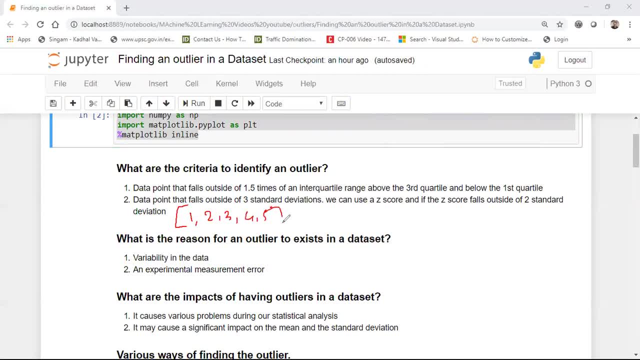 i'll just take a simple example like one, two, three, four, five, okay, and suppose i calculate the mean of this particular data set as three and my standard deviation is one. suppose i'm just considering it, guys, i'm not. i'm not calculating it, i'm just considering that. 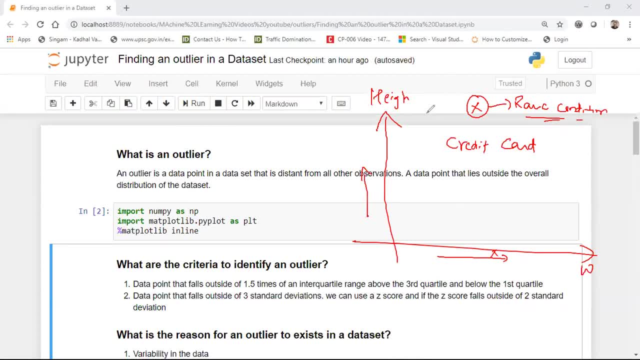 credit card fraudulent data, In that you'll be seeing that the weight is very, very high. You'll be seeing that some of the transaction will be very rare. You know, some of the transaction which is just like an, you know fraudulent data will be very rare, And that is what is. 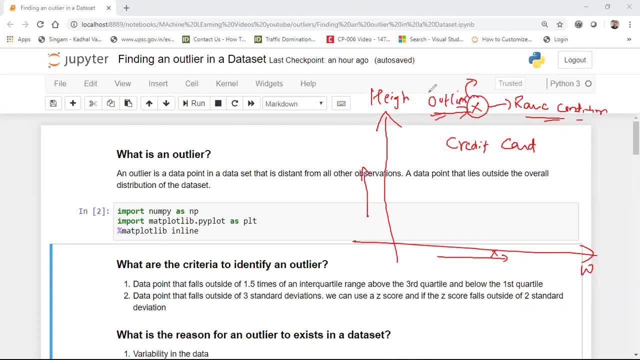 the most important outlier, data right. So there are various ways to handle this kind of outliers and this kind of outliers that are rarely present, If I take the example of height and weight. Okay, So they are different ways. In this particular video, we will be 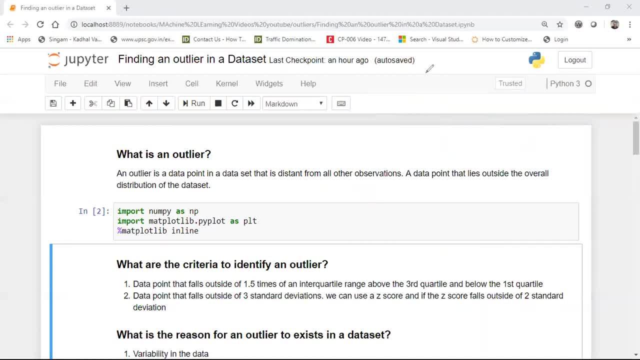 specifically seeing that, suppose, in a data set due to human error, there are some data that has got captured as an outlier. How do we find that particular outlier? How do we fix that? Okay, So initially, to begin with, I'm going to import some of the libraries. 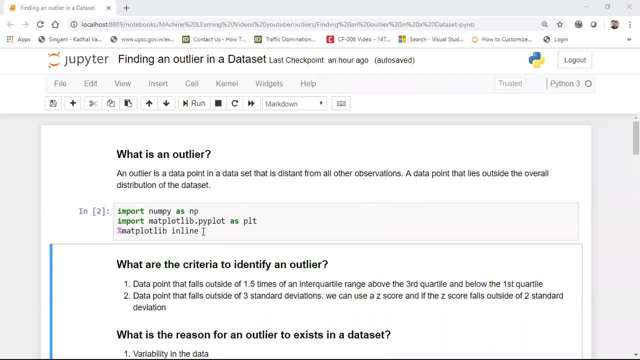 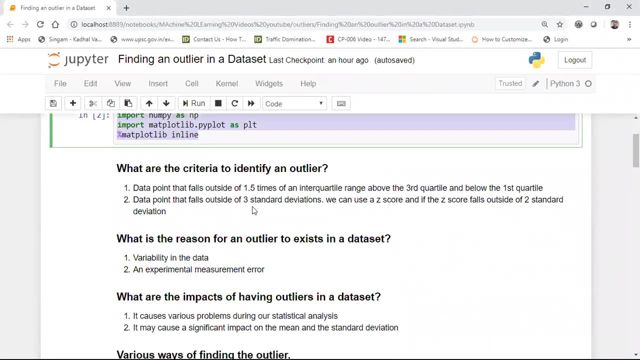 like NumPy, Pandas and Matplotlib. Sorry, Pandas is not there. NumPy and Matplotlib will be sufficient. Now what are the criteria to identify an outlier? See in this particular video, I'm going to show you two different techniques. One is with the help of something. 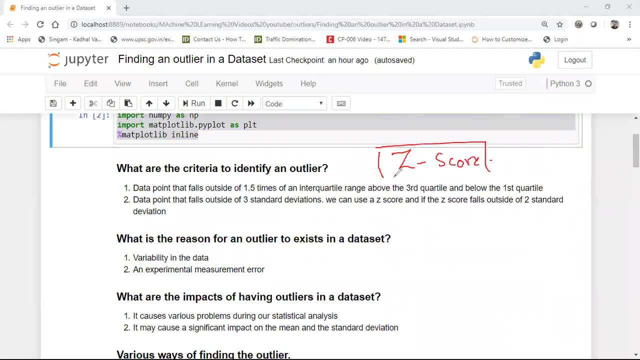 called a Z score. If you know about standard normal distribution, I think Z score will be very, very easy for you. This again, anyhow, I'll be explaining what is the Z score. Then the next thing is something called as intercontinental range. Okay, So we are going to discuss these two techniques. 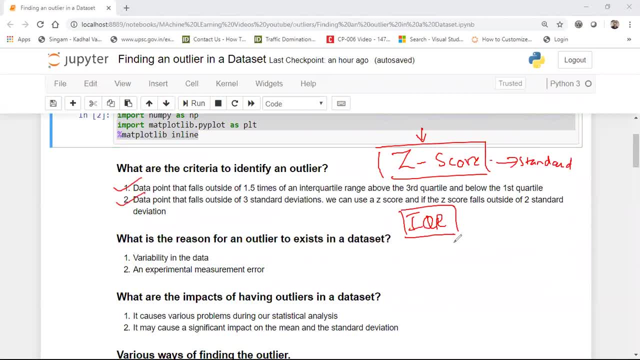 The first one is basically the intercontinental range. The second technique is something like a Z score. Okay, Now, what exactly is Z score? that we need to understand. Always remember, guys, whenever we have some data set. let me just take one feature, and I have some data. 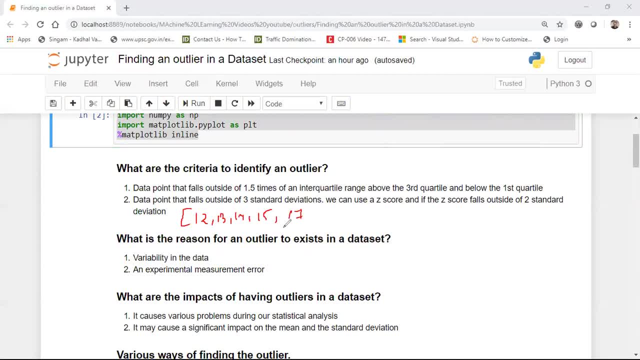 set like 12,, 13,, 14,, 15,, 17, or let me just clear this. Suppose- I'll just take a simple example- like one, two, three, four, five, Okay, And suppose I calculate the mean of this particular data set as three and my standard deviation. 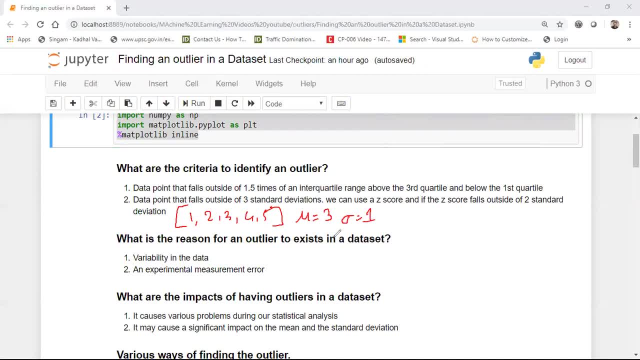 is one Suppose. I'm just considering it, I'm not calculating it, I'm just considering the mean will be three and standard deviation will be one. Now if I want to convert this distribution into a standard normal distribution, wherein the first property of standard normal distribution 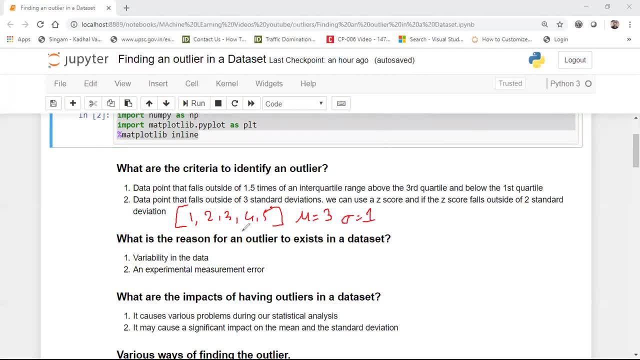 mean will be three and standard deviation will be one. now, if i want to convert this distribution into a standard normal distribution, wherein the first property of standard normal distribution is that mean is equal to 0 and standard deviation equal to 1.. so in order to convert this, we usually 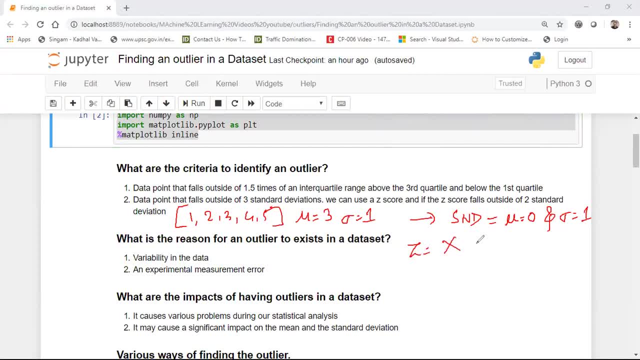 apply a z score formula which is something like x minus. this x is basically my all. my observation: i'll be considering minus mean by standard deviation. okay, this is how the z score is basically calculated and z score basically says that. in what standard deviation? whether in the 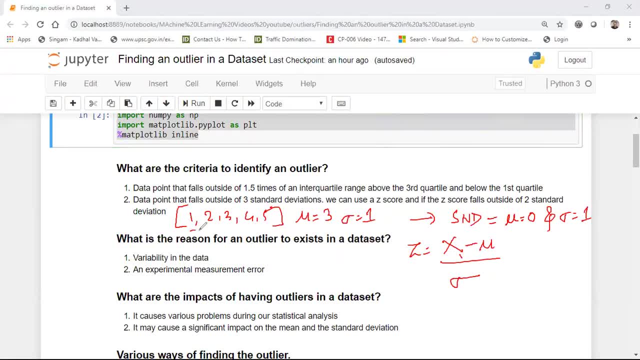 first standard deviation or in whether in the second standard deviation this particular data set actually falls into. and always remember, guys, in a standard normal distribution, right, if i have some kind of standard normal distribution, this center point is basically my mean, this is my first standard deviation, this is my second standard. 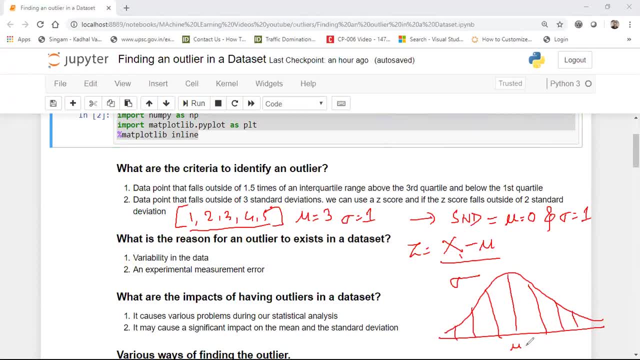 deviation. this is my third standard deviation and anything away from this, anything, any data that falls after this third standard deviation, are basically considered as my outliers. okay, as my outliers. so suppose i have this particular data set and suppose, if i apply this z score formula in this particular data set, if this z score formula fall within the standard deviation of three, 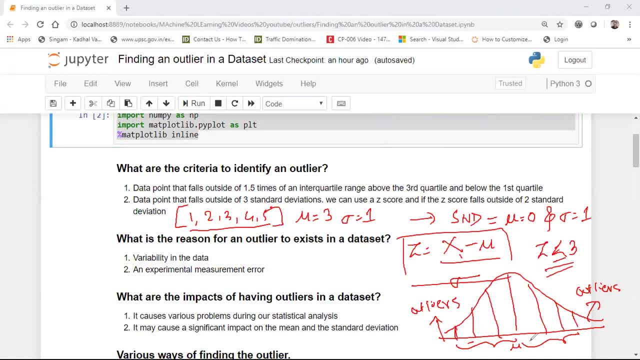 okay, within this three standard deviation, third standard deviation- that time i will be considering that this particular data set is not an outlier. if any data set falls away from this particular third standard deviation, then i will be considering as an outlier, and that is how we are going to. 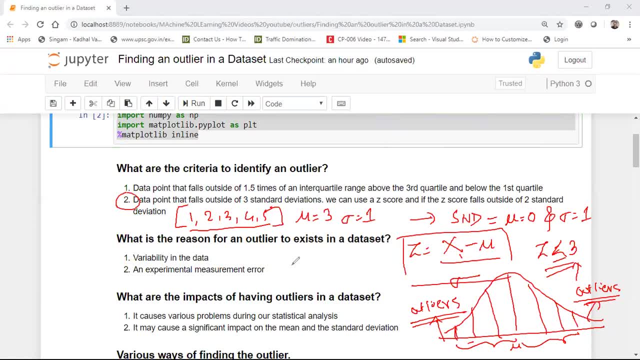 perform the second step, z score, what we'll do? suppose i have given a feature like f1 and this is having all the features of the data set and i have this particular data set, which is not an outlier, features like this. I will go and see that- which all features over here, which all values. 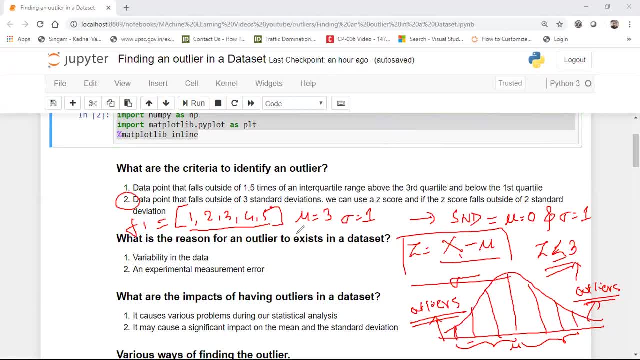 over here fall within the third standard deviation, Suppose. if it does not follow, or if it does not fall within the third standard deviation, then I'm going to consider that particular value as my outlier. Simple, very easy, Okay. So this is how a Z-score works. Now the other. 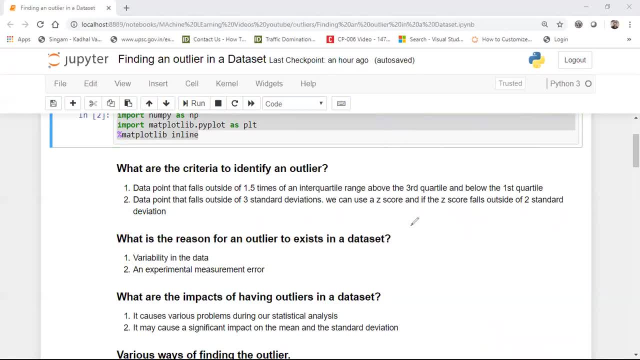 technique is something called as intercontinental range, That is, IQR In intercontinental range. there are some steps involved. What we do is that you should need to know what is percentiles Okay, Before understanding intercontinental range. Now suppose, guys, I have this features. 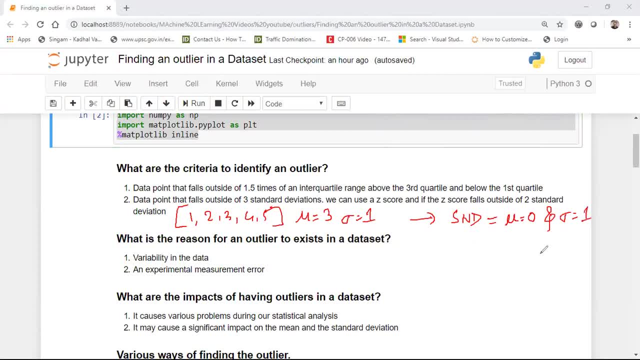 is that mean is equal to zero and standard deviation equal to one. So in order to convert this, we usually apply a Z score formula, which is something like X minus. this X is basically my all, my observation. I'll be considering minus mean by standard deviation. 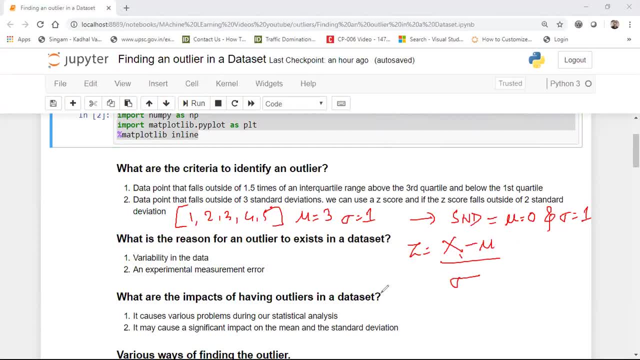 Okay, This is how the Z score is basically calculated and Z score basically says that in what standard deviation, whether the first standard deviation or whether in the second standard deviation this particular data set actually falls into. and always remember, guys, in a standard normal distribution, right, If I have some kind of standard normal distribution. 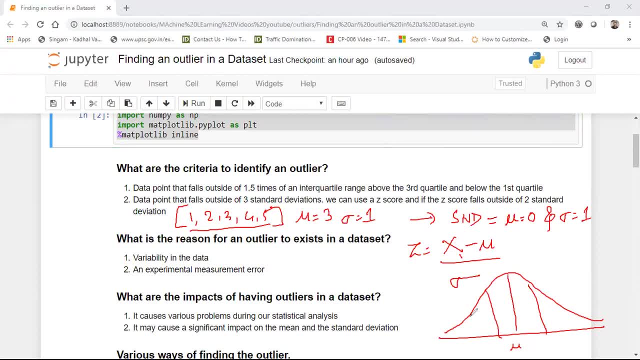 this center point is basically my mean. this is my first standard deviation, This is my second standard deviation, This is my third standard deviation and anything away from this, anything, any data that falls after this third standard deviation, are basically considered as my outliers. Okay, As my outliers, So suppose I have this particular data set. 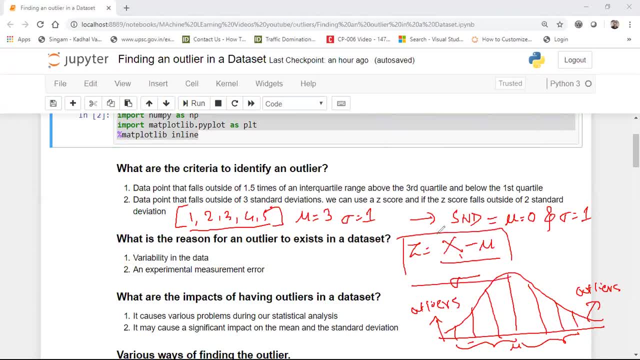 and suppose, if I apply this Z score formula in this particular data set, if this Z score formula fall within, Okay, Within the standard deviation of three, okay, Within this three standard deviation, third standard deviation, that time I will be considering that this particular data set is not an outlier. 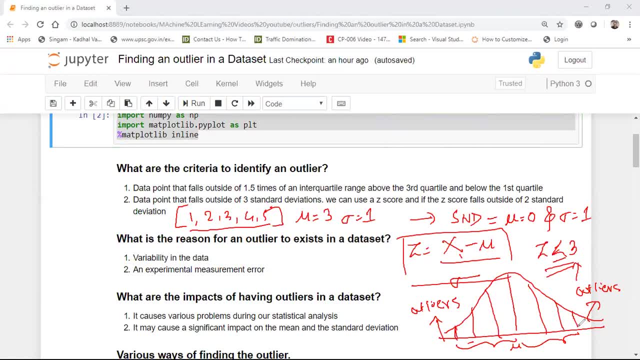 If any data set falls away from this particular third standard deviation, then I will be considering as an outlier, And that is how we are going to perform the second step. just score what we'll do. Suppose I've given given a feature like F1, and this is having all the features. 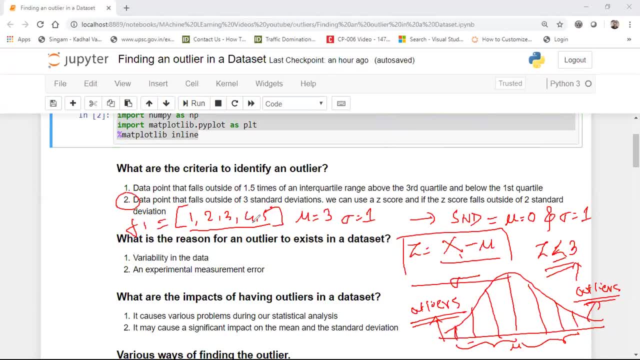 like this: I will go and see that which all features over here, which all values over here Fall within the third standard deviation, Suppose. if it does not follow, or if it does not fall within the third standard deviation, then I'm going to consider that particular. 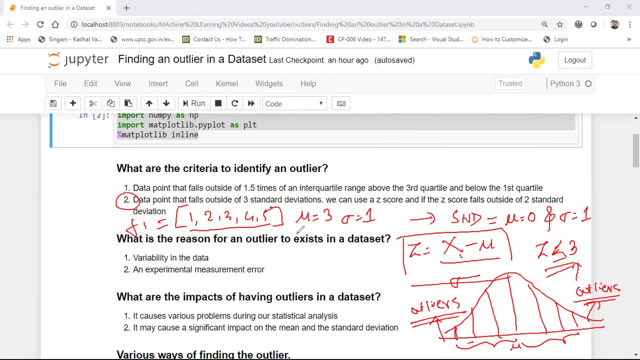 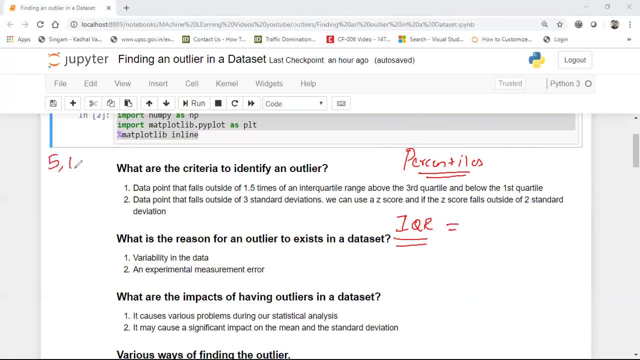 Now suppose, guys, I have this features, like I have some values like five, six, seven, and I have one too, Okay, So, in order to find a percentiles, what we do is that we will try to. you know, suppose I have some more numbers like four, nine, eight, over here. 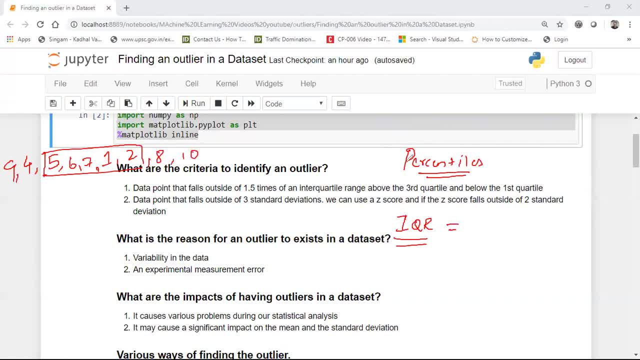 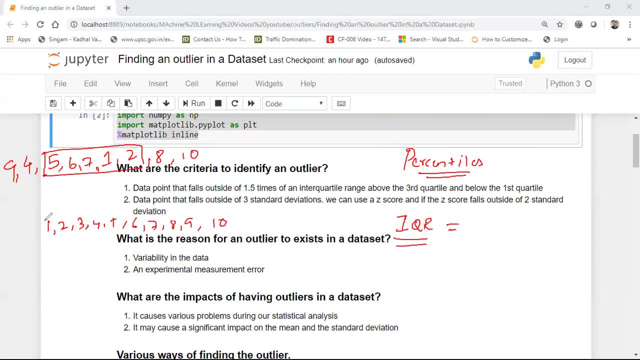 to find out the person bass. what we'll do is that first of all, sorting mechanism will and 10 after sorting right. what we do is that suppose, if I consider one, this one is nothing but my 0th percentile. this basically indicates that they are no. 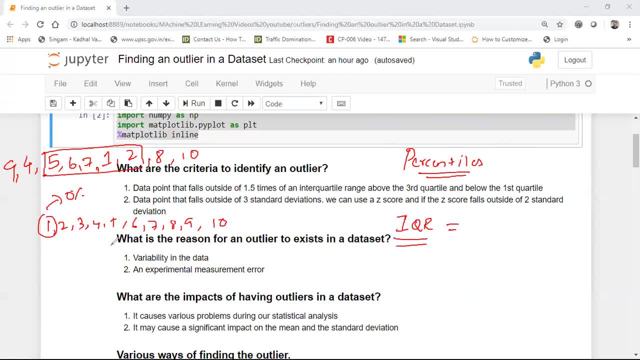 number. they are zero number, zero percentage of number less than one that are smaller than one, sorry, that are lesser than one. okay, there are zero numbers, and that is true because I don't have any numbers less than one way. suppose, if I consider tell two, since I have ten numbers over here, two will. 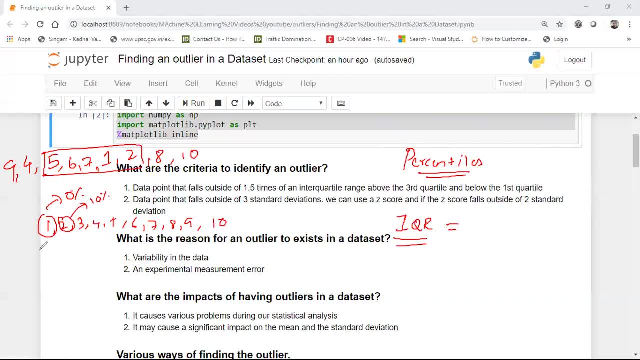 basically become my ten percentile number. that basically means that ten percent of the total numbers over here in this particular distribution are less than two under trade. ten percent of this numbers are only one right. I have only one number which is less than two, which is nothing. but from this total ten numbers it is actually ten percent. okay, now if I 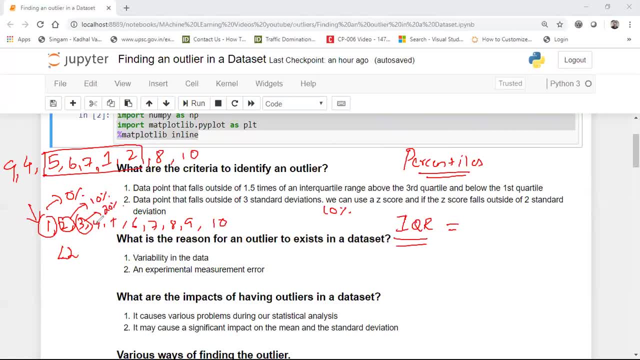 could consider three over here. this becomes my twenty percent. that basically indicates that twenty percent of my number is less than three. eighty percent of number, 80 percent of the number in this distribution is less than two. what I am saying is what I am saying, that I don't. 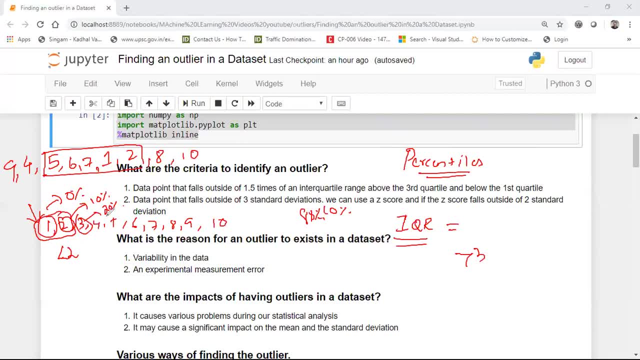 distribution is greater than three. right, So similarly, four. four will actually be my 30%. that basically indicates that 30% of this distribution, in this particular distribution, is less than four. 70% is greater than four or greater than equal to four. Okay, That. 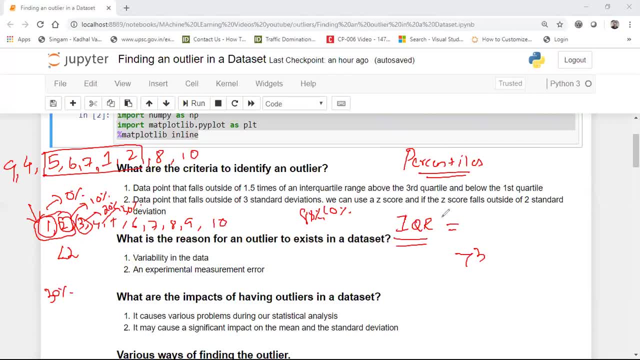 is how it is indicated. Now in intercontinental range, the most numbers that we'll be focusing on will be 25 percentile, 75 percentile, And then we calculate 75 percentile values in this distribution. Suppose, if I'm taking this particular distribution as an example, we 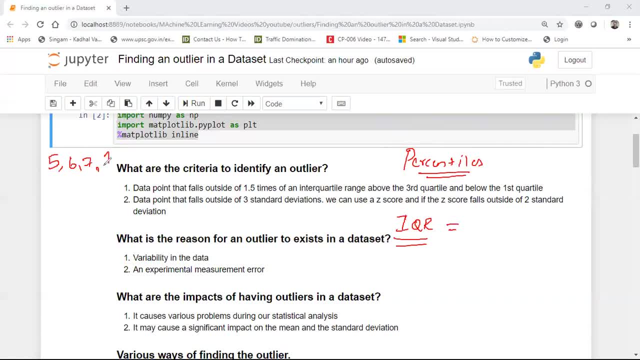 like, I have some values like five, six, seven, and I have one, two. Okay. So, in order to find out percentiles, what we do is that we will try to. you know, um, uh, suppose I have some more numbers like four, nine, um, eight over here and 10.. Okay, So, if I want to find, 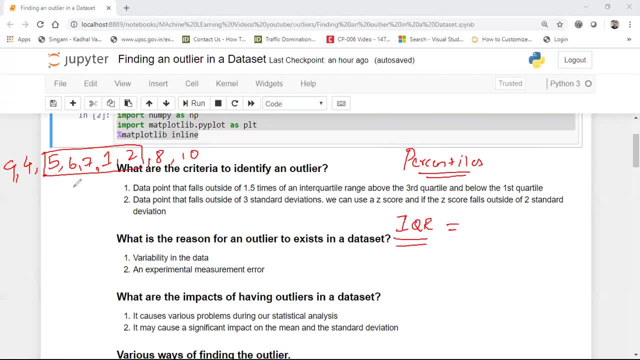 out the percentiles. what we do is that we will try to. you know, um, uh, suppose I have some more numbers like four, nine, um eight over here and 10.. Okay, So if I want to find out the percentiles, what we'll do is that, first of all, sorting mechanism will happen. 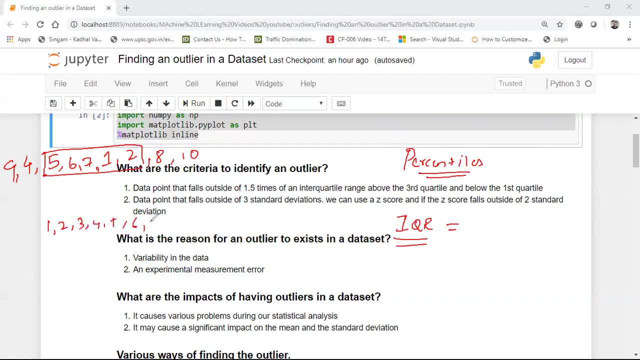 in this numbers, So it will become sorted: One, two, three, four, five, six, seven, eight, nine, 10.. After sorting right, What we do is that suppose, if I consider one, this one is nothing but my zero percentile. This basically indicates that they are no number, They are. 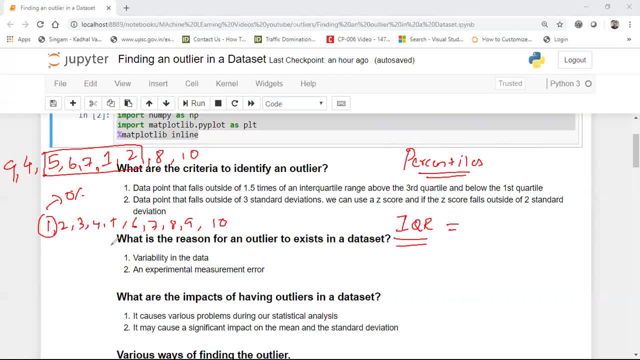 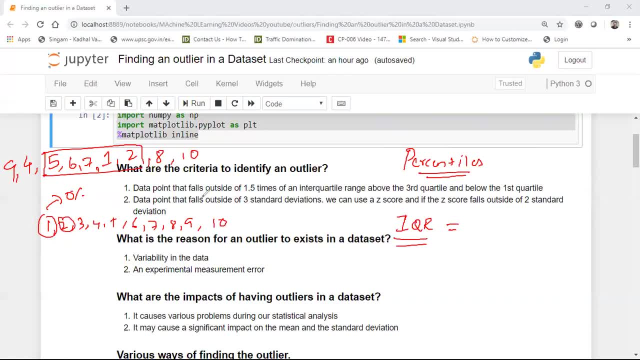 say, let's say let's say less than one. Suppose, if I consider two, since I have 10 numbers over here, two will basically become my 10 percentile number. That basically means that 10% of the total numbers over here in this particular distribution are less than. 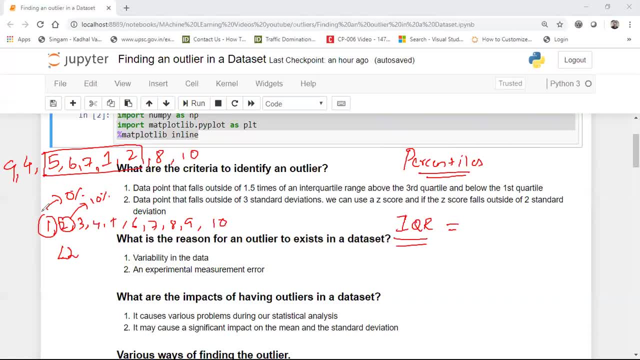 two Under 10%. of this numbers are only one. right, I have only one number which is less than two, which is nothing, but from this total 10 numbers, It is actually 10%. Okay, Now, if I consider three over here, this becomes my 20%. That basically indicates that 20%. 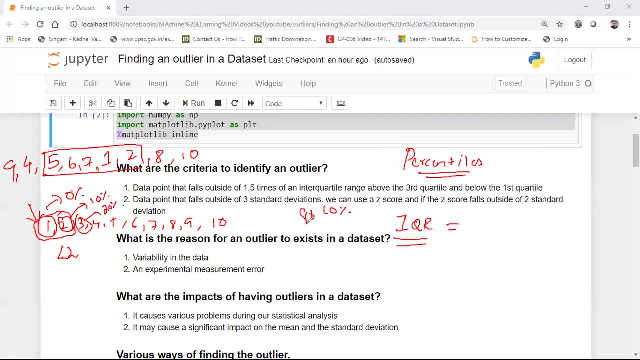 of my number is less than 3. 80% of number: 80% of the number in this distribution is greater than 3, right? so similarly, for 4 will actually be my 30%. that basically indicates that 30% of this distribution in this particular distribution is less than 4. 70% is greater than 4 or greater. 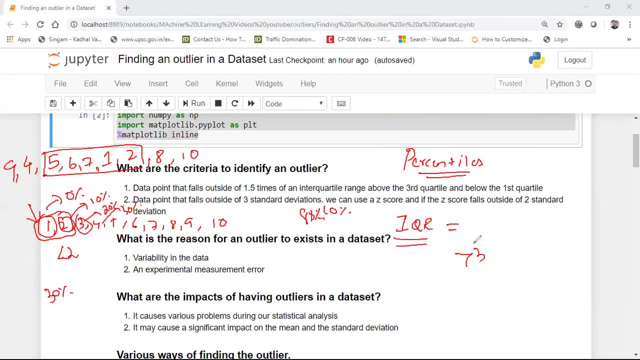 than equal to 4. okay, that is how it is indicated. now, in intercontinental range, the most numbers that will be focusing on will be 25 percentile, 75 percentile, and then we calculate 75 percentile values in this distribution. suppose, if I am taking this particular distribution as an 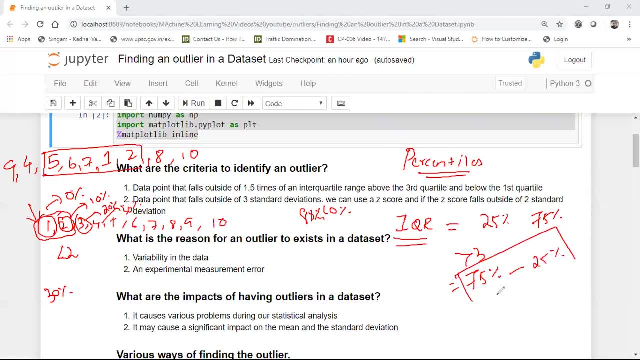 example, we subtract it with 25 percentile and that is basically my IQR, that is basically my intercontinental range, that is basically that 75 percentile number, whatever I am get, and if I am subtracting with 25 percentile number, that is basically my intercontinental. 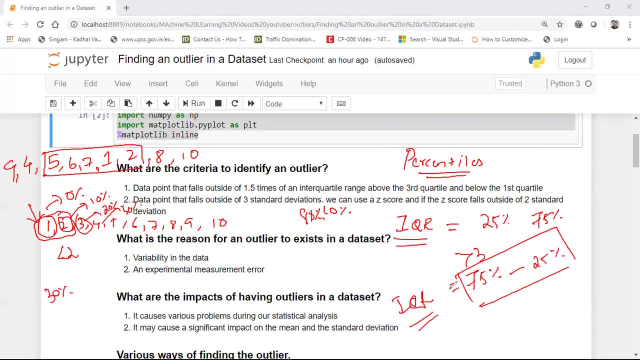 okay, simple. now how to detect an outlier after finding an outlier IQR value, that I will just discuss in a moment. okay, so this was two techniques: one is Z score and one is intercontinental range. after this, what I am going to explain you is that what? 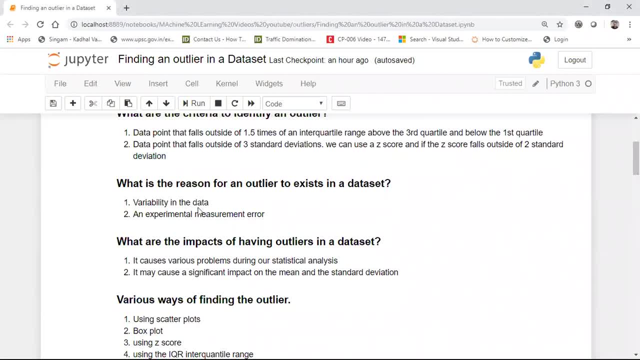 are the reasons for an outlier to exist in a data set? first of all, variability in the data. the second reason is that there is an experimental measurement error or it may be some human error. they are not calculated it properly. what are the impacts of having an outlier in a data set? they are various impacts, because the statistical analysis that you 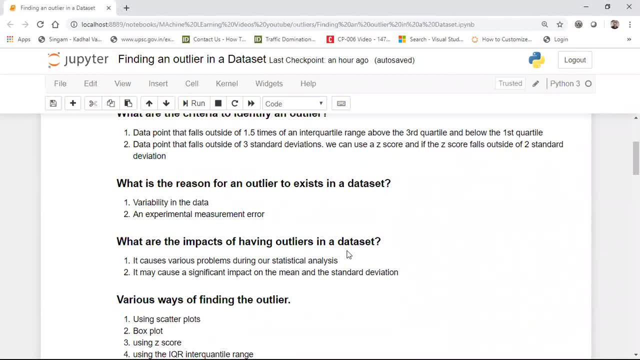 will be doing if there are a lot of outliers that are present. Okay, And it may affect that particular analysis. okay, and it may also have some more problems when we are actually trying to calculate the mean and the standard deviation. always remember, guys, due to the outliers, your mean and standard deviation may change a lot and that is the. 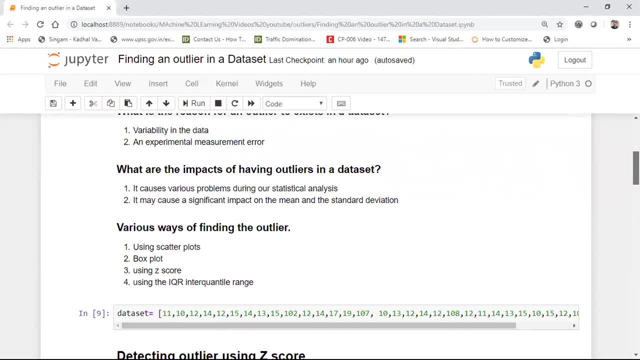 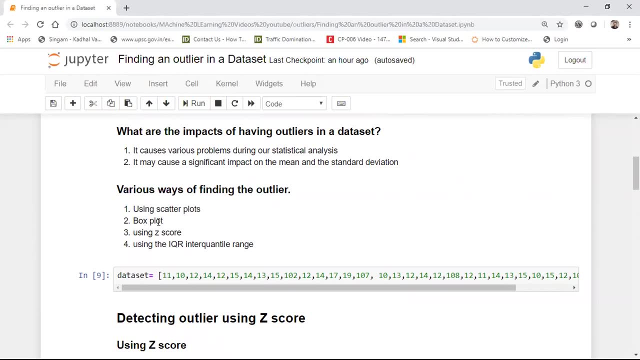 reason that these are some of the impacts that will may happen if our outlier is present. various phase of finding the outlier. one way is basically by using scatter plot. the second way is something like box plot. scatter plot is just like distribution of X and Y, if I 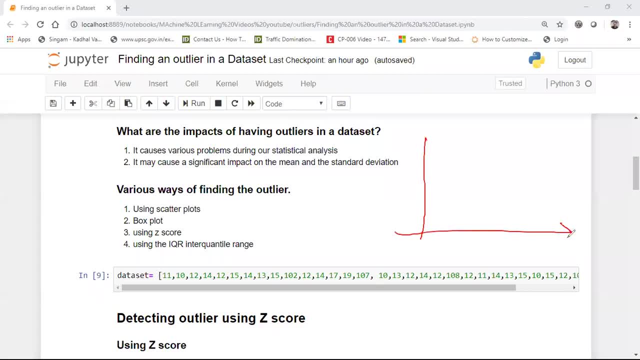 just show you X and Y. just remember this. suppose this is my X axis and Y axis. suppose I have some of the distribution which is somewhere here. okay, but there will be some points that will be plotted here. so these are my outliers and by using a scattered plot I will be able 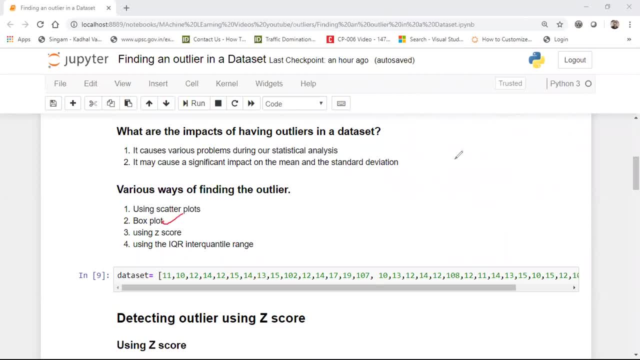 to see: okay. similarly, if I come up with box plot, box plot is nothing, but I'll be having this kind of boxes. you know, this will be my 25 percentile, this will be your 50 percentile, this point will be a 75 percentile. Okay. 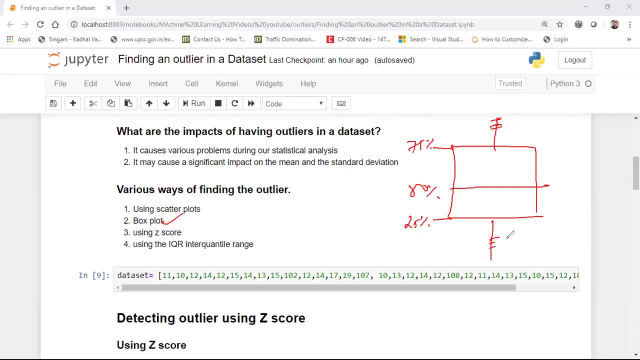 So this is one example of box plot, but again I'll explain. I just have calculated IQR. after finding IQR, how do I determine the outlier? first of all, let me just try to show you how to do with that, with the Z score, with the help of a code. now suppose, imagine that this: 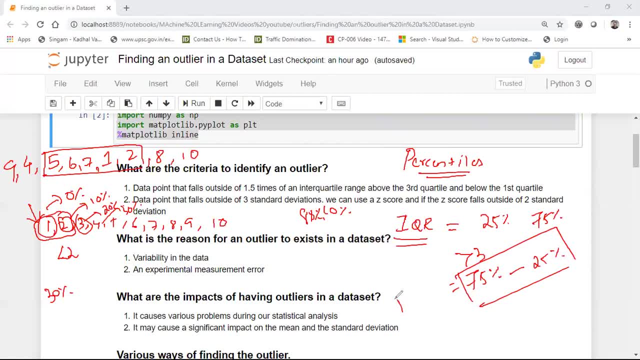 subtract it with 25 percentile And that is basically my IQR. That is basically my intercontinental range. That is basically that 75 percentile number, whatever I'm get, And if I'm subtracting with 25 percentile number, that is basically my intercontinental. 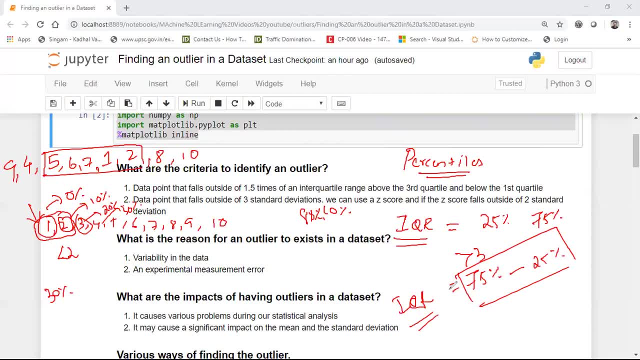 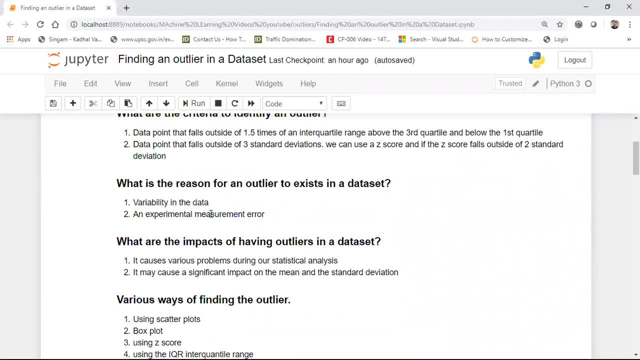 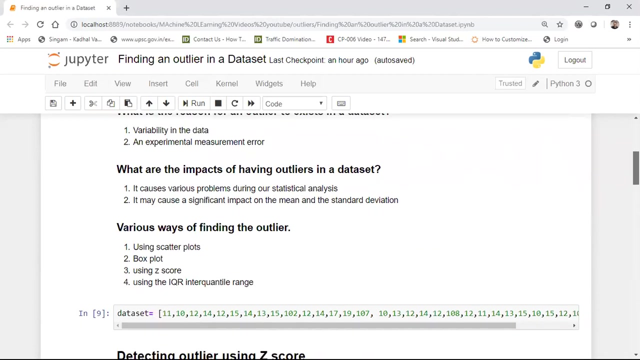 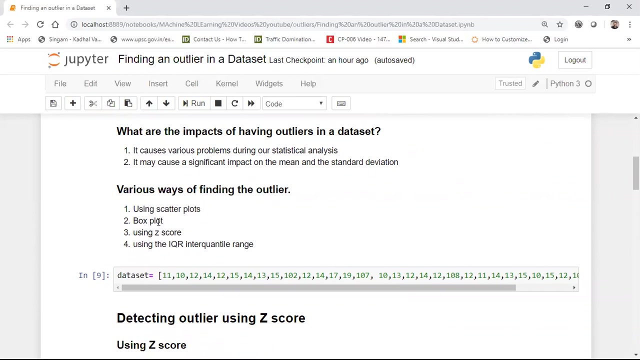 張 바의 may change a lot, and that is the reason that these are some of the impacts that will may happen if our flight is present various phase of finding the outlier. one way is basically by using scatter plot. the second way is something like box plot. uh, scatter plot is just like distribution of x and y. 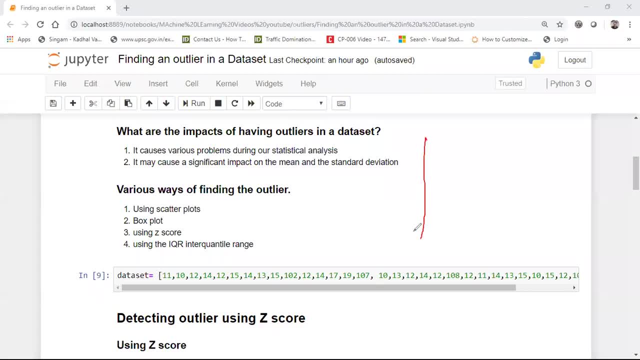 if i, if i, if i just show you x and y, just remember this. suppose this is my x axis and y axis. suppose i have some of the distribution which is somewhere here. okay, but there will be some points that will be plotted here. so these are my outlines and by using a scattered plot, i will be able to see. 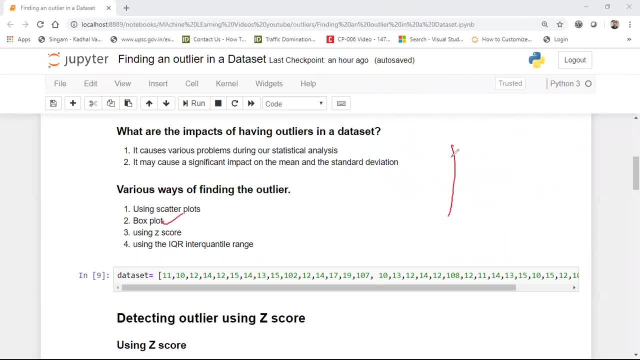 okay now, similarly, if i come up with box plot, box plot is nothing, but i'll be having this kind of boxes. you know this, this, this, this will be my 25 percentile, this will be your 50 percentile, this point will be a 75 percentile and anything above this over here will be your outliers. you. 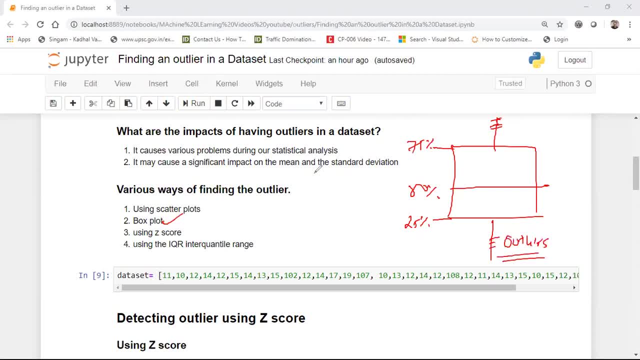 know outliers. okay, so this is one example of box plot. but again i'll explain. i just have calculated. i just have calculated the outliers and then i will be able to see how much of the outliers are IQR. After finding IQR, how do I determine the outlier? First of all, let me just try to show. 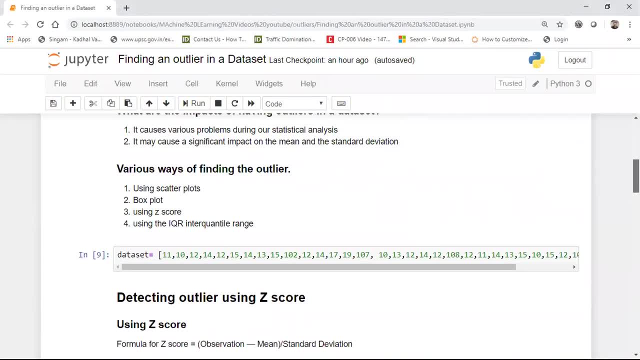 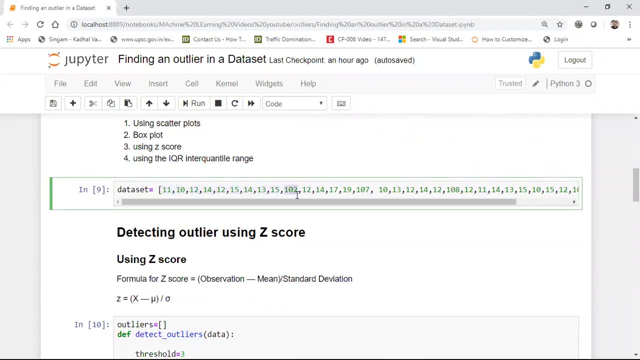 you how to do with that, with the Z score, with the help of a code. Now suppose, imagine that this is my data set over here: some values like 11, 10,, 12,, 14,, 12,, 15,, 14,, 15.. And you observe some of 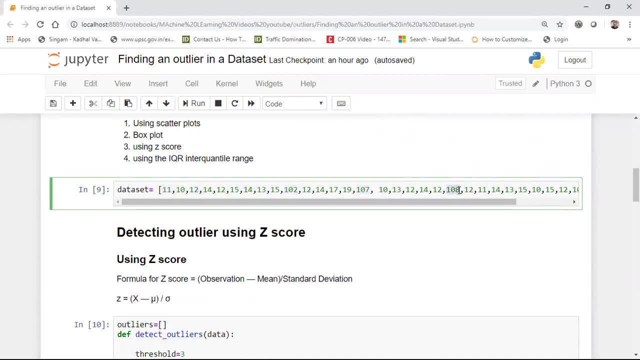 the numbers I have: 102,, 107,, 108. And by just seeing this particular data set, you may come into a conclusion that 102,, 107, and 108 may be an outlier because these values are higher when compared to the other distribution. but how to do it mathematically that we need to understand how. 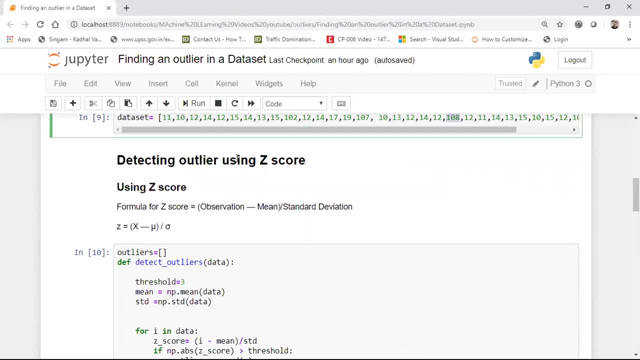 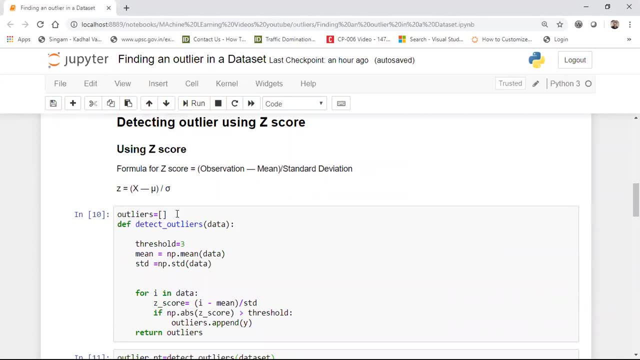 to do with the help of Python right Now: detecting outliers using Z score. First, I'm going to consider Z score, So remember Z score. the formula is X minus mu by standard deviation. So here I've created my outlier as my list, Okay, And I'm creating a function which will detect the outlier. 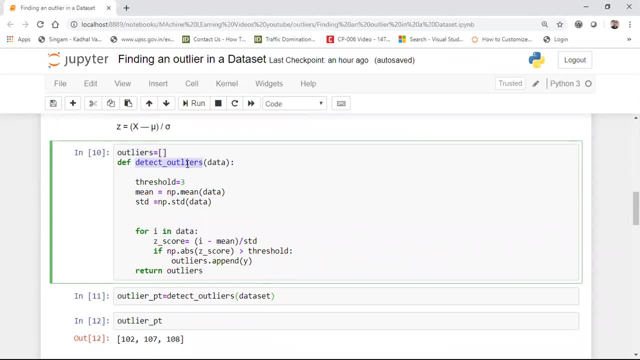 and to detect the outlier with the help of Z score. First of all, I need to find out the Z score value. Okay, So, uh, the threshold value. I'm keeping it as three. That basically means that within third standard deviation, if my data is falling, I'm going to consider, I'm not going. 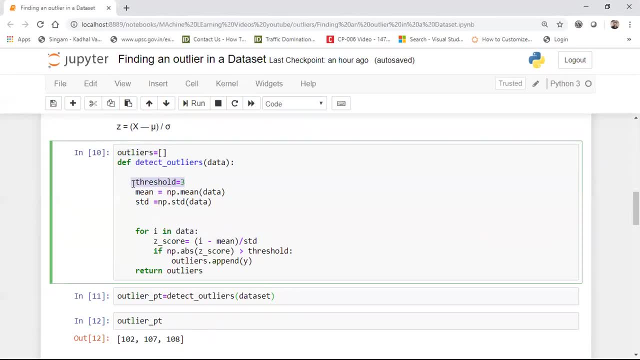 to consider that as an outlier. If it is falling away from the third standard deviation, then I'm going to consider it as an outlier. So first I'm going to compute the mean and standard deviation, because I need the mean and standard deviation based on this formula, And then I'm going to put 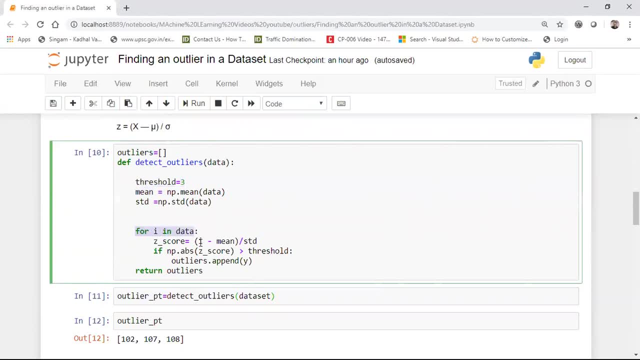 a for loop in my data set. for each and every data set I'm going to subtract, I'm going to apply this particular formula and try to find out the Z score If that particular value is. uh, whatever Z score value is coming over here Once I get this particular Z score value, if that Z score value. 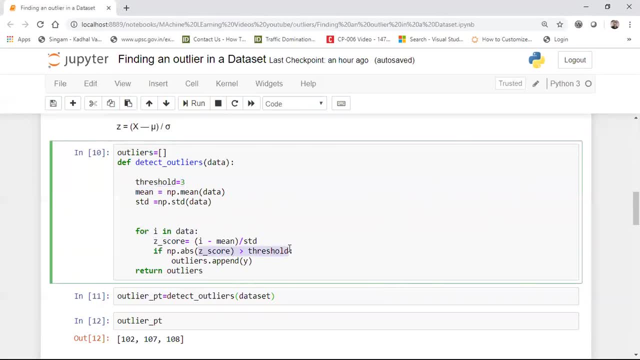 is greater than the threshold value. Okay, If the Z score value is greater than threshold value, that basically means if it is falling away from the third standard deviation, if you are calculating the Z score, if it is more than three, I'm going to append that particular Y value, that particular. 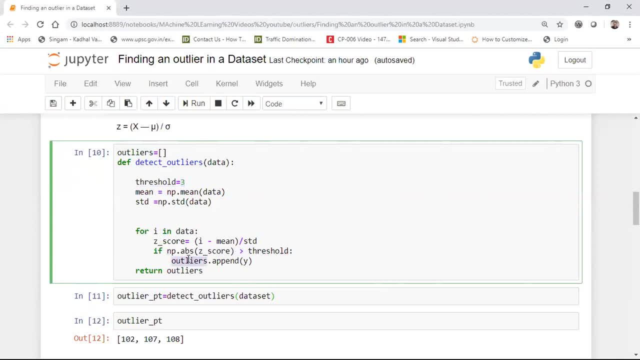 Y value in my outliers. Okay, That is what I'm actually trying to do. Sorry, It should not be Y. I'm going to append my I value in this particular Z score value. So I'm going to append that particular particular outliers. So this particular I value indicates that it does not fall within the third. 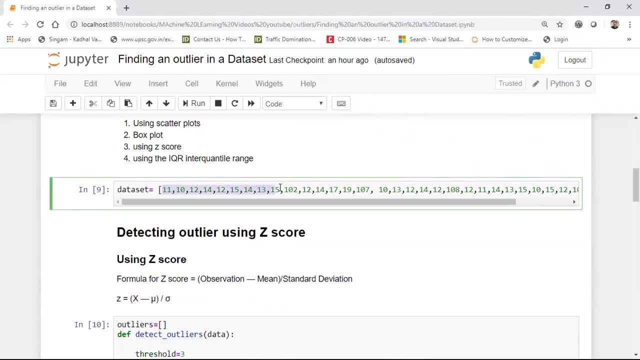 is my data set over here, some values like 11, 10, 12, 14, 12, 15, 14, 15, and you observe some of the numbers I have: 102., 107, 108, and by just seeing this particular data set, you may come into a conclusion that 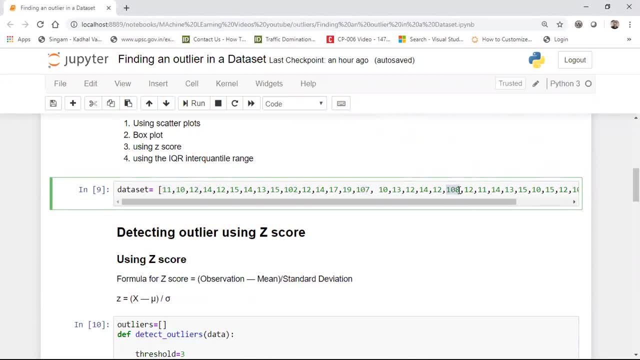 102, 107 and 108 may be an outlier because these values are higher when compared to the other distribution. but how to do it mathematically that we need to understand how to do with the help of python right now, detecting outliers using Z score. first, I'm going to consider 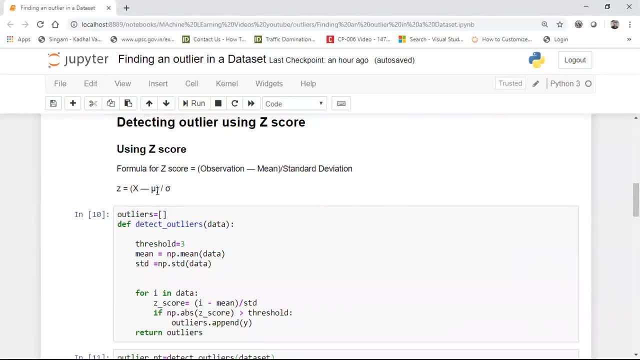 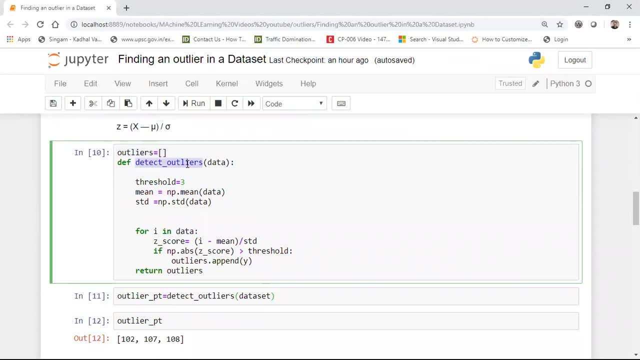 Z score. so remember Z score. the formula is X minus mu by standard deviation. so here I've created my outlier as my list, Okay, And I'm creating a function. I'm going to detect the outlier, and to detect the outlier with the help of Z score. first, 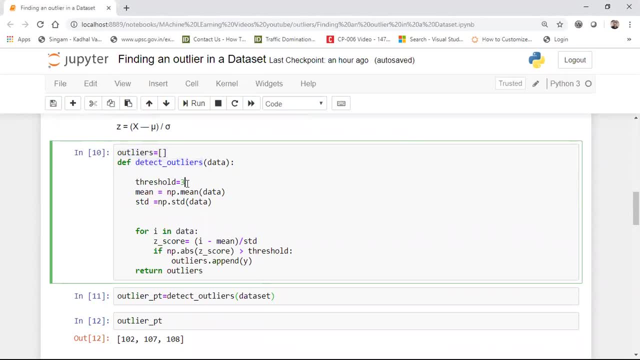 of all, I need to find out the Z score value. okay, so the threshold value, I'm keeping it as three. that basically means that within third standard deviation, if my data is falling, I'm going to consider. I'm not going to consider that as an outlier if it is falling away from. 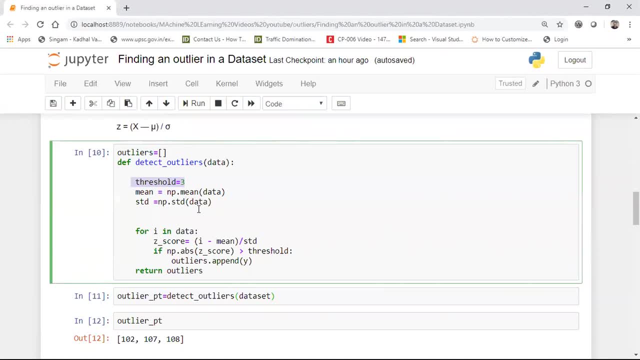 third, standard deviation. then I'm going to consider it as an outlier. So first I'm going to compute the mean and standard deviation, because I need the mean and standard deviation based on this formula. Then I'm going to put a for loop in my data set. for each and every data set I'm going 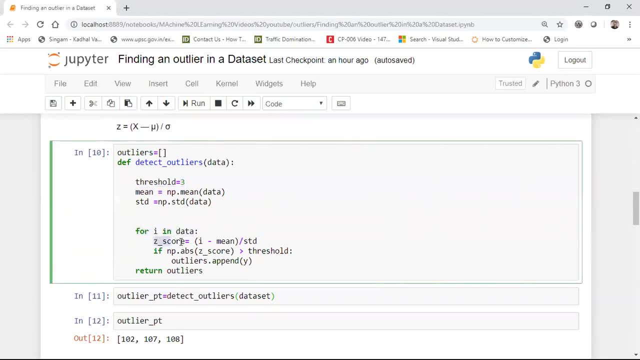 to subtract. I'm going to apply this particular formula and try to find out the Z score if that particular value is. whatever Z score value is. coming over here once I get this particular Z score value, if that Z score value is greater than the threshold value, okay. if the Z score value is greater than threshold value, that basically means if it. 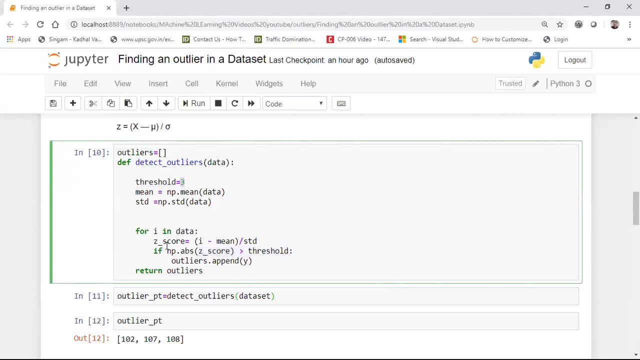 is falling away from the third standard deviation if you are calculating the Z score, if it is more than three, Okay, Okay, So I'm going to put a particular Y value, that particular Y value, in my outliers. Okay, That is what I'm actually trying to do. 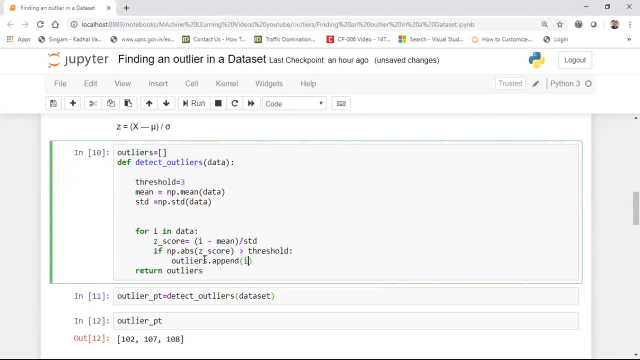 It should not be Y. I'm going to append my I value in this particular outliers. This particular I value indicates that it does not fall within the third standard deviation. for adding that in my outliers list. Okay, And similarly, to go and check for each and every you know values in this particular data. 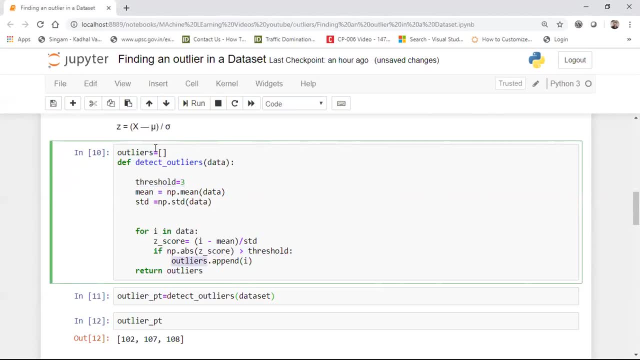 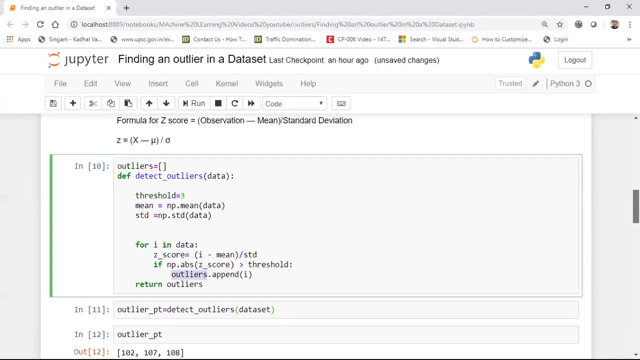 standard deviation. So I'm adding that in my outliers list, Okay, And similarly, it will go and check for each and every uh you know, uh values in this particular data set, in this particular data set. it'll go and check Now, uh, this, this was about this particular function. 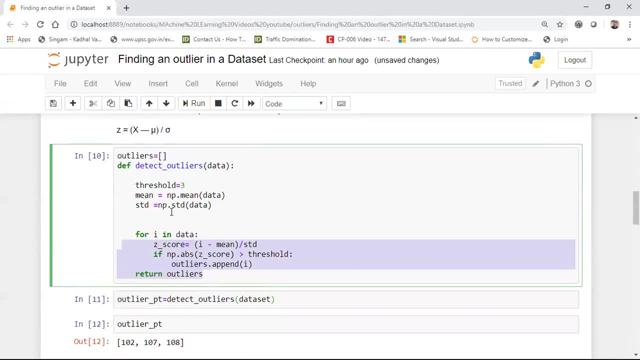 guys. Uh, I'm trying to see for each and every values that are present in that particular data set whether that falls in the outlier or not. if it does not fall in the outlier or not, I'm going to retrieve that particular record and append it in my outlier list. So here it is, I am. 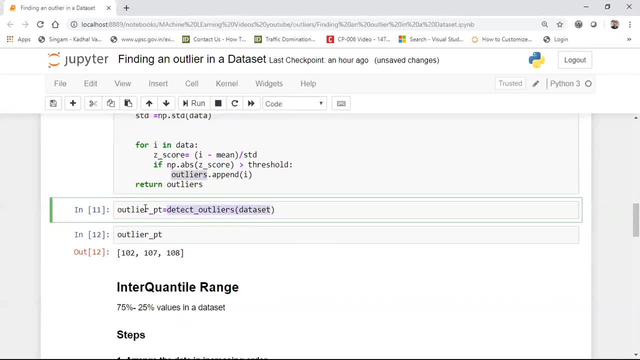 applying this particular function. I am giving my data set And as soon as I see my outlier point, I'm getting a hundred and 207, a hundred. Now you can see perfectly They have got the outlier by just using a simple method of Z score. If it is falling within the third standard deviation. 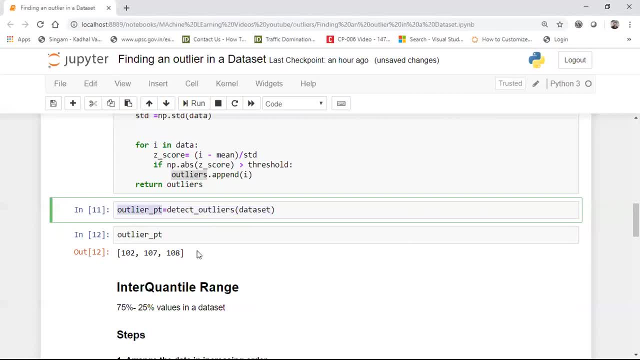 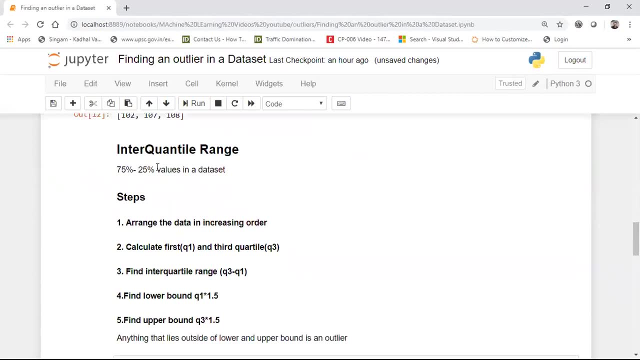 I'm considering it. If it is not falling, I'm just considering that as an outlier. Okay, Now the next point. I'm going to go with the interquantile range. Interquantile range is my 75 percentile value minus 25 percentile. First of all, they are some steps in interquantile. 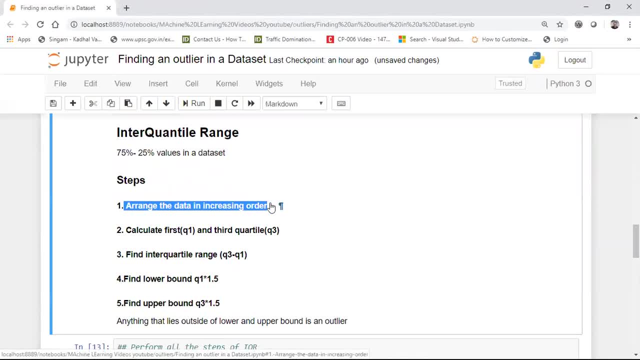 range. First of all, we arrange the data in increasing order. Okay, Basically, in the sorted order, we calculate the first quantile and the third quantile. This is basically my 25 percentile and this will basically be my 75 percentile. Then we find out the difference from the third. 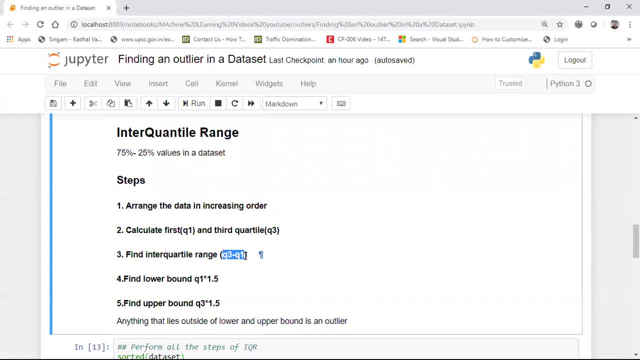 quantile, that is, my 75 percentile and the 25 percentile. And finally, I found out the lower point. Lower bound value basically means that, uh, below what point? below what point in that particular data set I'm going to consider that belongs to an outlier? and higher bound, or the upper bound, basically means that from 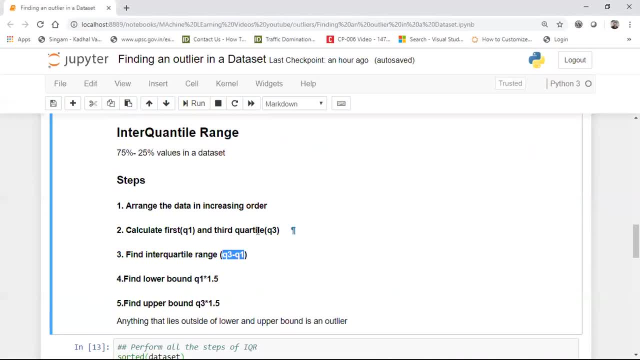 the third quantile. okay, what value I have to consider in the top that uh? that particular data set does not belong within that particular uh interquantile range. So I'm going to calculate my lower bound value and the upper bound value in order to calculate. what I have to do is. 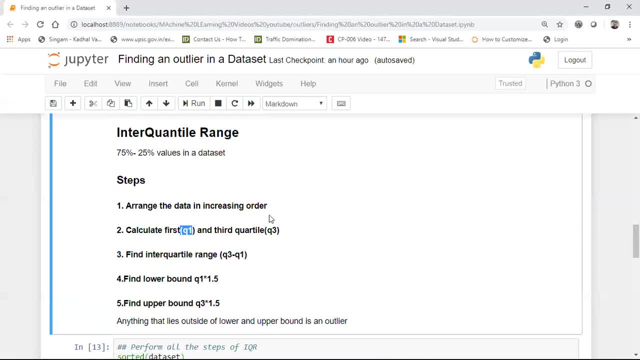 that whatever first quantile I'm getting, I have to multiply with 1.5, whatever third quantile I'm getting, I'm going to multiply with 1.5. simple, this many steps are there and anything that lies outside of lower and upper bound is basically an outlier. Now, 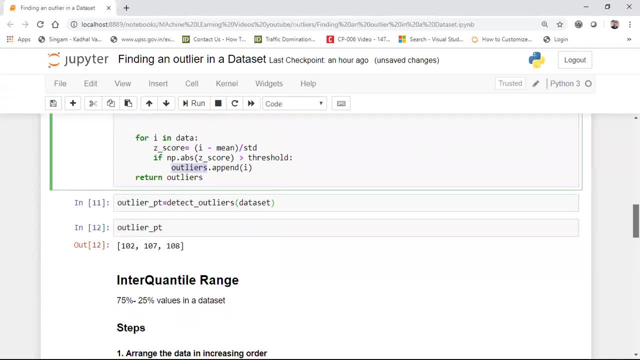 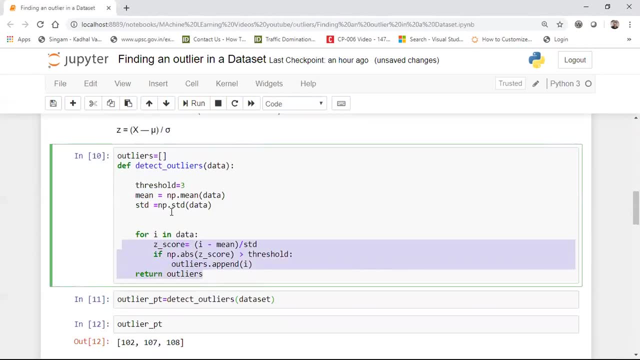 set in this particular data set. It'll go and check. Now, this was about this particular function. guys, I'm trying to see for each and every values that are present in that particular data set whether that falls in the outlier or not. If it does not fall in the outlier, I'm going to retrieve that particular record and append. 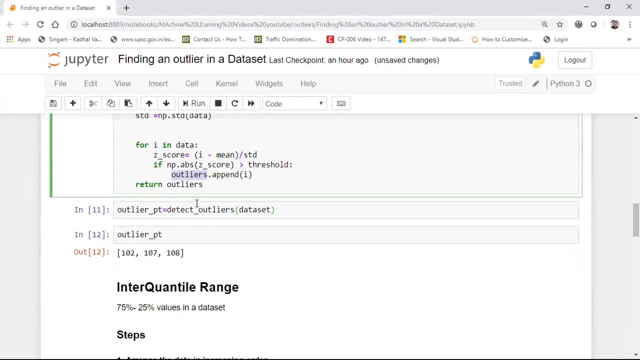 it in my outlier list. So here it is. I am applying this particular function, I am giving my data set and as soon as I see my outlier point, I'm getting hundred and two hundred and seven hundred. now you can see perfectly. they have got the outlier by just using a simple method. 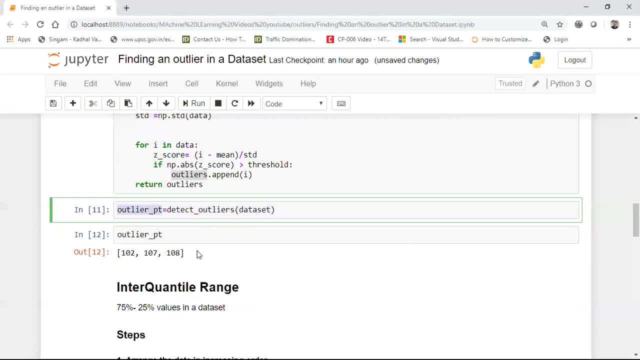 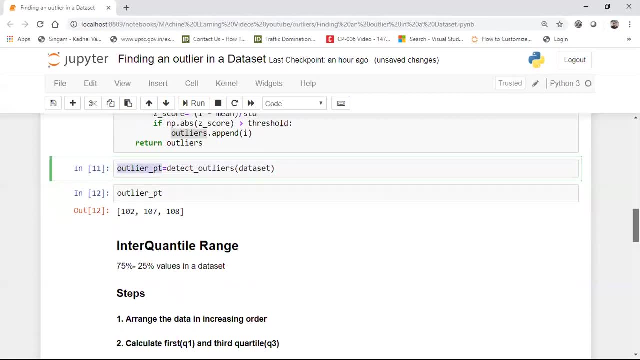 If it is falling within the third standard deviation. I'm considering it is not falling and just considering that as an outlier. Now the next point I'm going to go with the interquantile range. interquantile range is basically my seventy five percentile value minus twenty five percent. 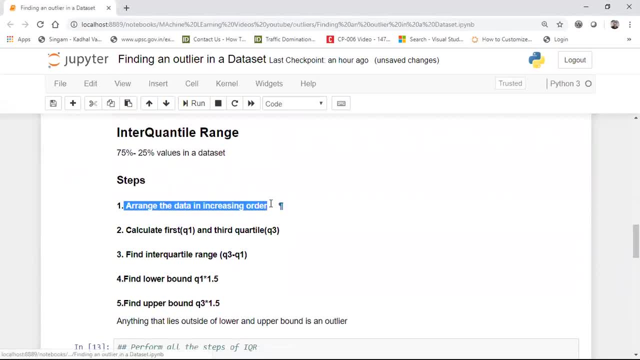 First of all, there are some steps in interquantile range. First of all, we arrange the data in increasing order. Okay, Basically, in the sorted order, we calculate the first quantile and the third quantile. This is basically my twenty five percentile and this will basically be my seventy five percentile. 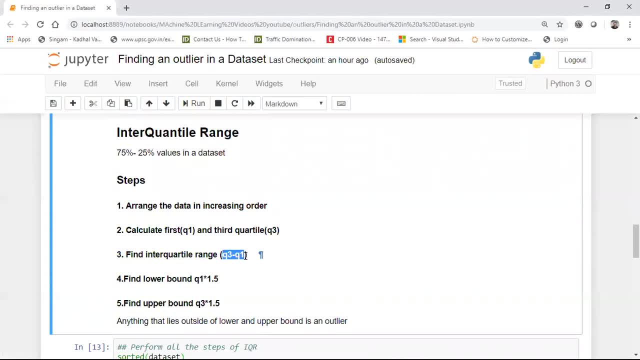 Then we find out the difference from the third quantile, that is, my seventy five percentile, and the twenty five percentile, And finally I find out the lower bound. lower bound value basically means that, below what point? below what point in that particular data set I'm going to consider that belongs. 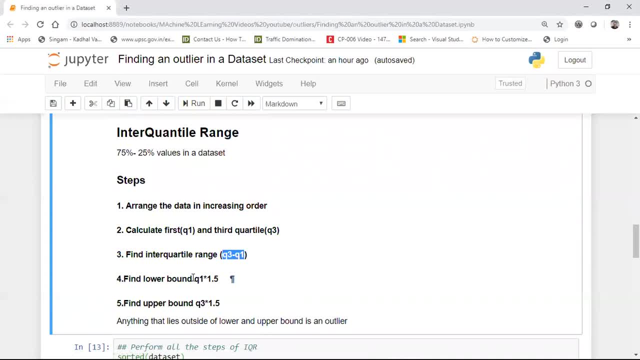 to an outlier and higher bound or the upper bound basically means that from the third quantile- Okay, What value I have to consider in the top? that that particular data set does not belong within that particular Interquantile range. So I'm going to calculate my lower bound value and the upper bound value in order to calculate. 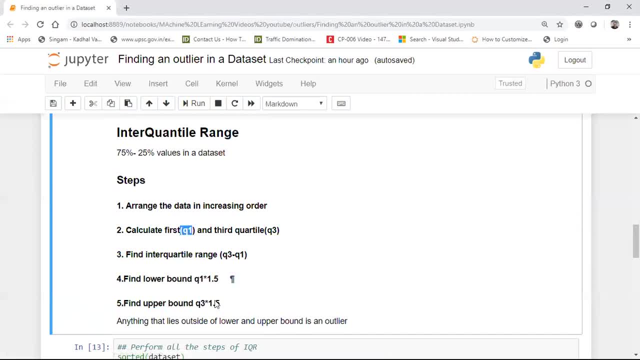 what I have to do is that whatever first quantile I'm getting, I have to multiply with one point five. whatever third quantile I'm getting, I'm going to multiply with one point simple. There's many steps out there and anything that lies outside of lower and upper bound. 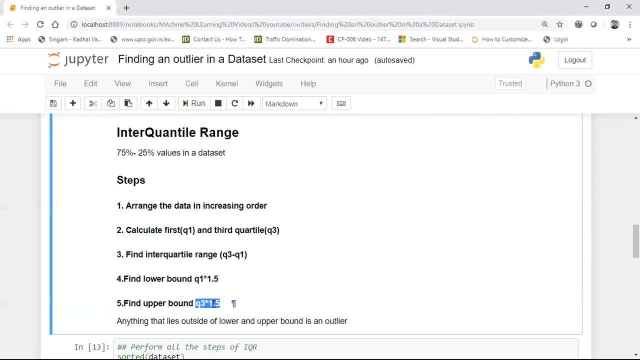 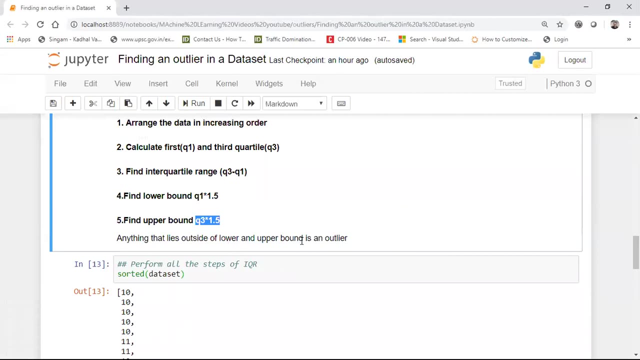 is basically an outlier. Now how I'm considering one point five and one point five That is based on the distribution pattern, most suitable value that we have actually found out. So for that reason, we are basically using so anything that lies outside of lower and 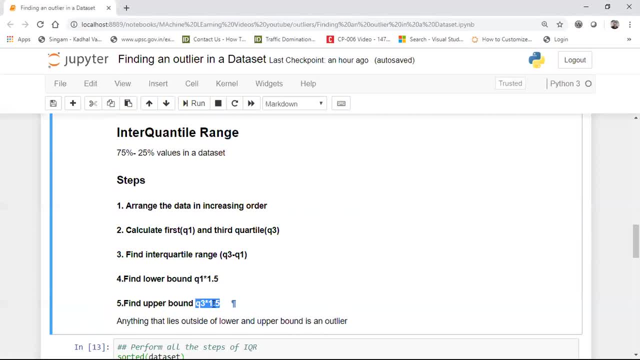 how I'm considering 1.5 and 1.5 over here. that is based on the distribution pattern. Most suitable value that we have actually found out for multiplying- that has been proved already- is 1.5.. Okay, So for that reason, you're basically using, so anything that lies. 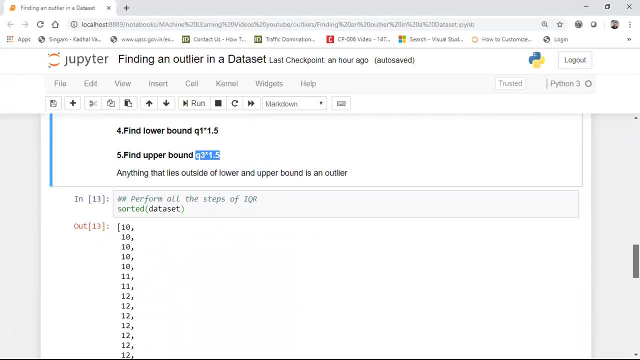 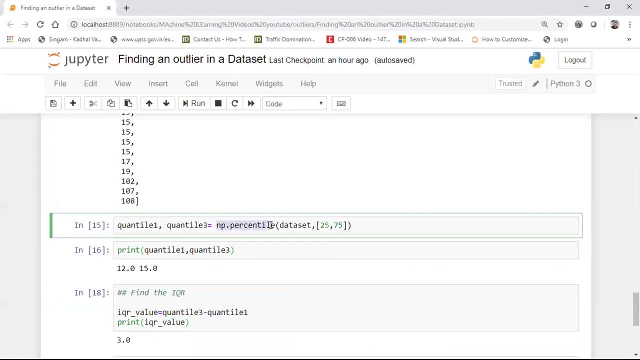 outside of lower and upper bound is basically an outlier. So this is the way how you can do the sorted. All this step by step. what I'll do is that I will basically use a function inside the numpy which is called as nppercentile. 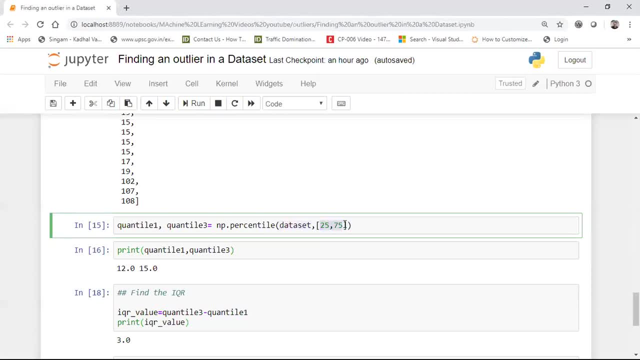 And here I'm going to give my data set and here I'm specifying that I need the 25 percentile value and the 75 percentile value. As soon as I do this, I'll be getting my lower bound over here and my upper bound. 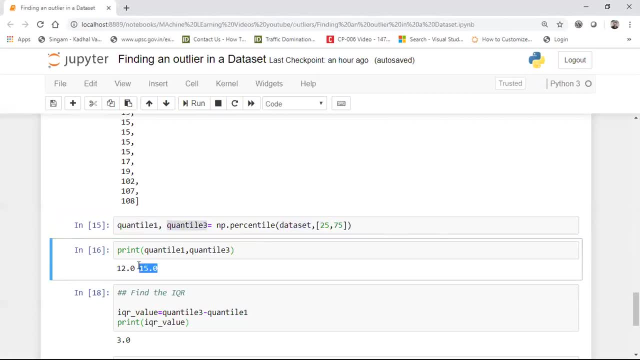 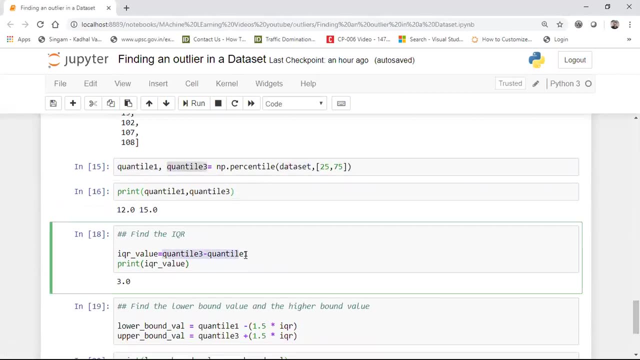 And if you see my lower and upper bound, this is basically 12.0 and 15.0.. And then I'll try to find out the difference between this. So here it is. I'll find out quantile 3 minus quantile 1.. 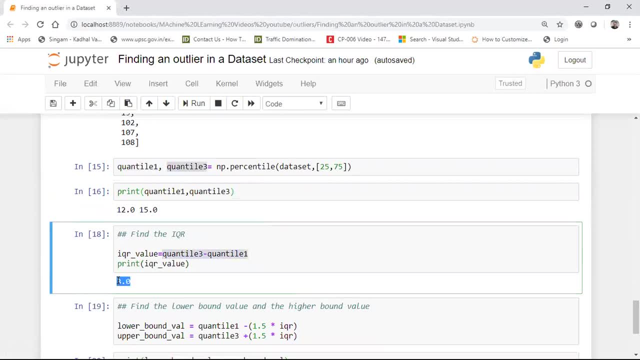 This is basically my 3 value, But still I need to find out what is my. you know the lower bound and the higher bound value which I'm considering after my step 4th and 5th. So for that I have to multiply with 1.5.. 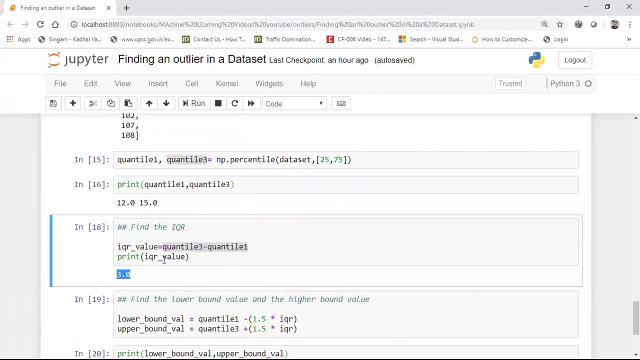 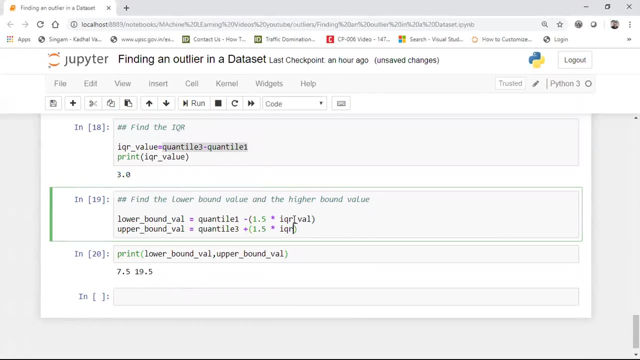 So I'll go down over here. Here is my IQR underscore value. So what I'm doing? I'm going to find out my lower bound value and the upper bound value. So, lower bound value: as usual, I said quantile 1.. 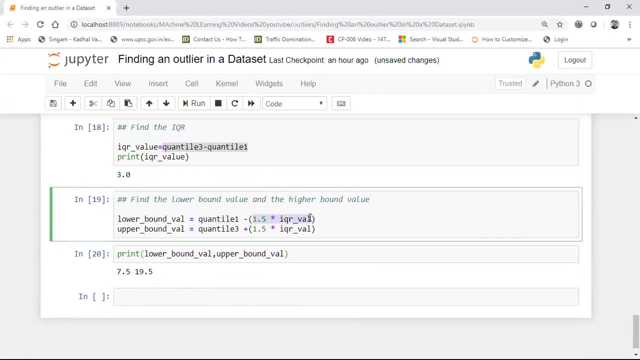 Minus 1.5 multiplied by IQR value, And upper bound. I'm saying that quantile 3 plus 1.5 multiplied by IQR underscore value. When I do this, this is my lower bound, This is my higher bound. 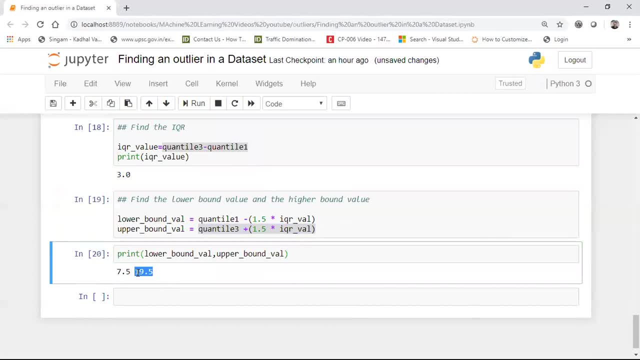 So anything, any values if it is away from this particular lower bound and upper bound, that is basically considered as an outlier. And this is how you can do: a very simple method by using IQR and the z-score, And you can find out the difference between the lower bound and the higher bound. 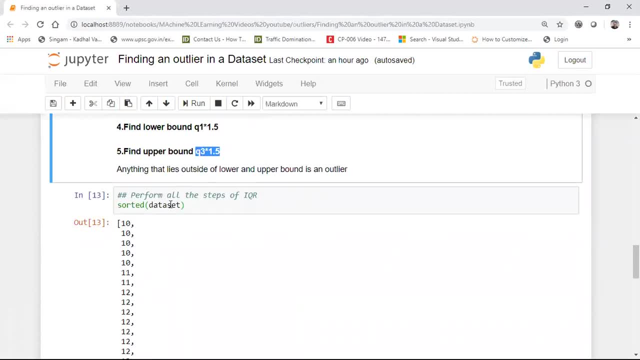 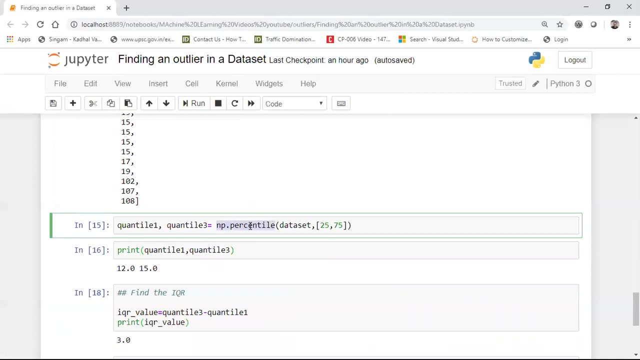 upper bound is basically an outlier. So this is the way how you can do the sorted. I don't want to do all this step by step. What I'll do is that I will basically use a function inside the numpy which is called as NP dot percentile, and here I'm going to give my data set and here I'm specifying that. 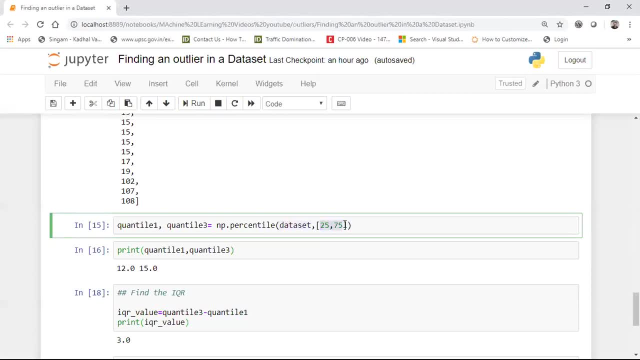 I need the 25 percentile value and the 75 percentile value. as soon as I do this, I'll be getting my lower bound over here And my upper bound, And if you see my lower and upper bound, this is basically twelve point zero and five point. 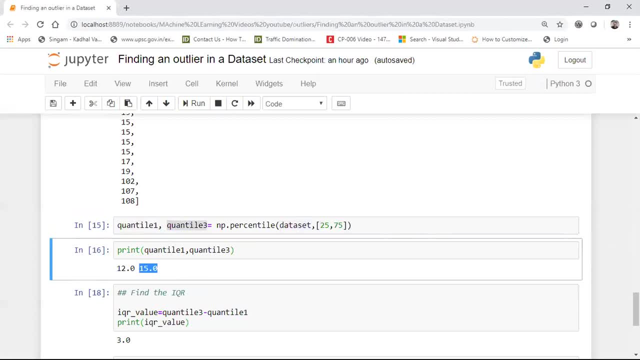 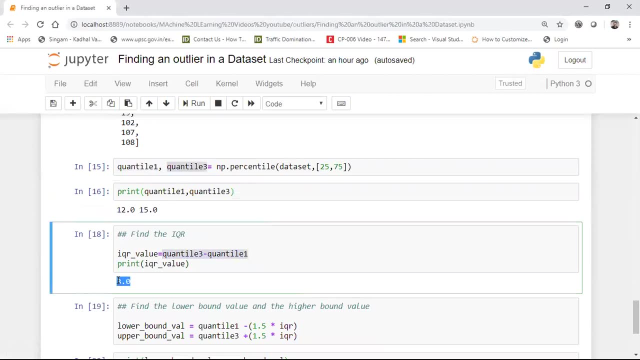 fifteen point zero, And then I'll try to find out the difference between this. So here it is, I'll find out. point three minus one. This is basically my three value. OK, but still I need to find out what is my. you know the lower bound and the higher bound. 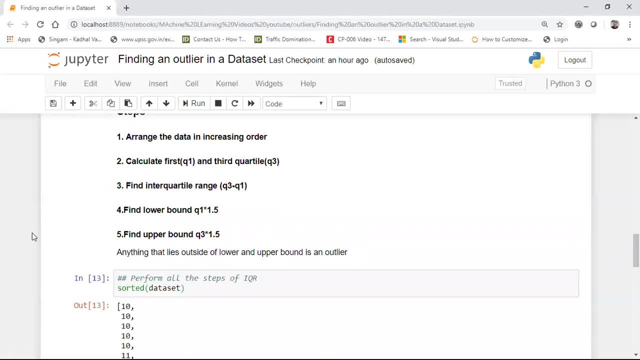 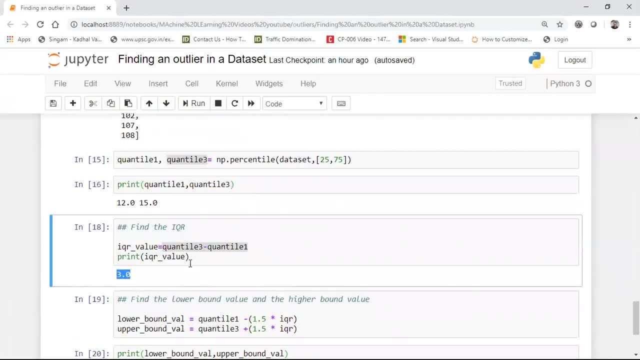 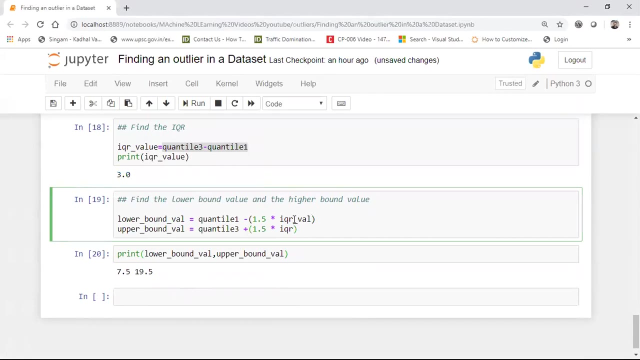 value which I'm considering after my step fourth and fifth. OK, Before that, I have to multiply with one point five. I'll go down over here. OK, Here is my IQR underscore value for what I'm doing. I'm going to find out my lower bound value and the upper bound value. 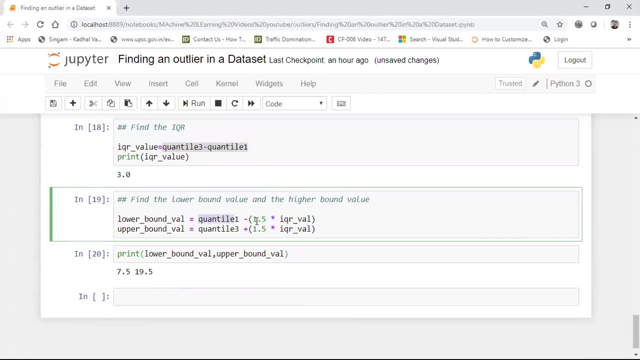 So lower bound value. as usual, I said quantile one minus one point five multiplied by IQR value and upper bound. I'm saying that quantile three plus one point five multiplied by IQR underscore value. When I do this, this is my lower bound, this is my higher bound. 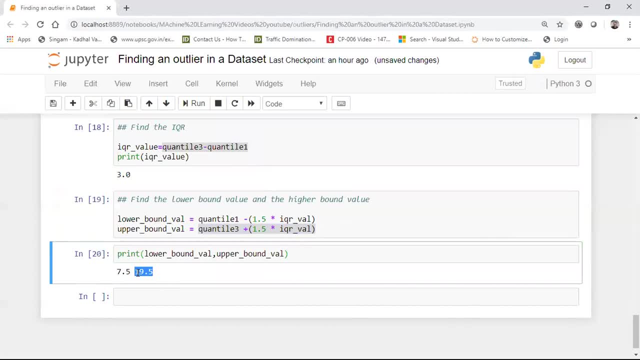 So anything, any values, If it is away from this particular lower bound and upper bound, that is basically considered as an outlier. And this is how you can do a very simple method by using IQR and Z score, and you can find out an outlier in a data set. 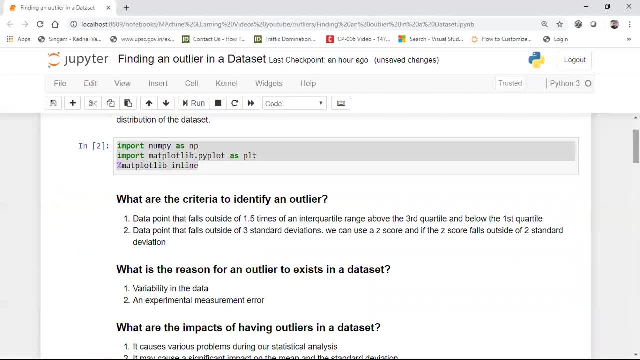 In my next video I'm going to take a very good example of a data set you know from a Kaggle competition, and then I'm going to show you how you can find out an outlier and how you can fix that outlier in that particular problem statement. 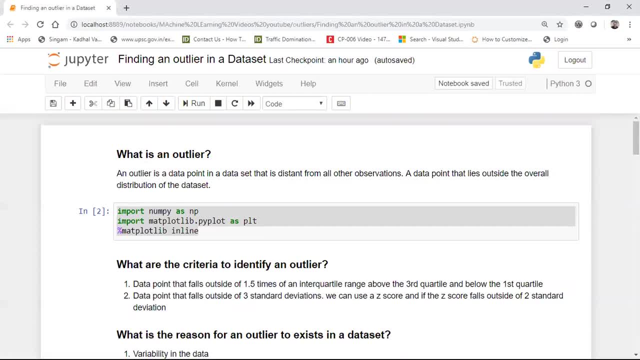 So I hope you like this particular video. Guys, please do subscribe to the channel if you are not already subscribed. Please share with all your friends who ever require this kind of help. And, yes, I'll see you all in the next video. Have a great day ahead. 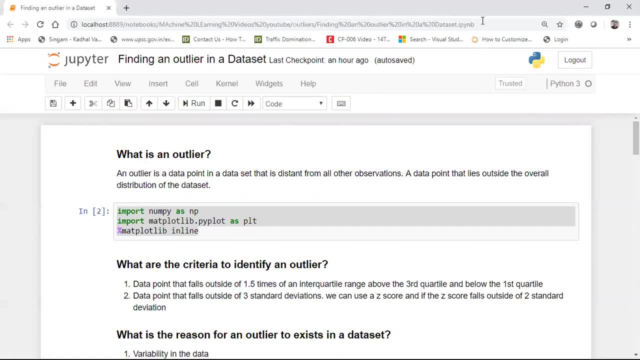 Keep on learning, Never give up. I'll see you all in the next video. God bless you all. Thank you One minute.